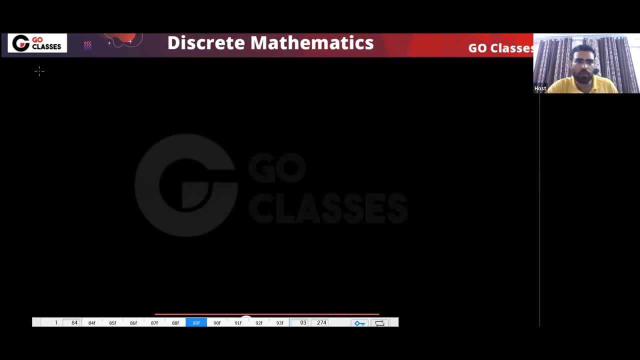 In propositional logic. what is the interpretation? Let's see. See in propositional logic, if I give you some expression, Like let me give you P or Q, Tell me, is it true or false This expression I am giving you, Is it true or false? 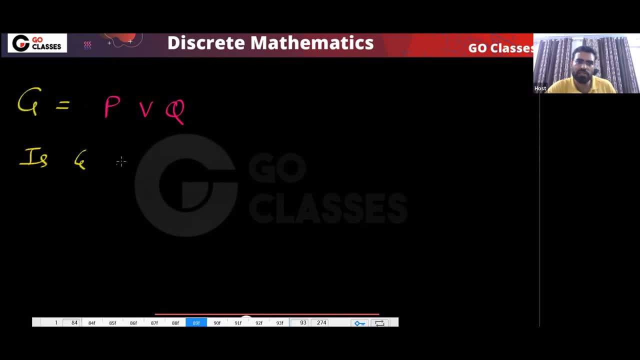 This is my question. Let me call it G. Is G true? Is G true or false? Tell me, If you want to find the truth value, then what will happen? Let's assume these are the variables. So if you want to find the truth value of this, then what do you need? 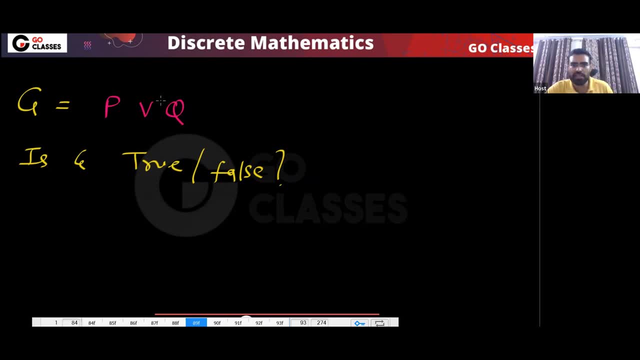 You need the truth value of P comma Q, right? Yes or no? So that's the point. If you want to find the truth value of this, then the question is: what is the truth value of P comma Q? You need the truth value of P comma Q. 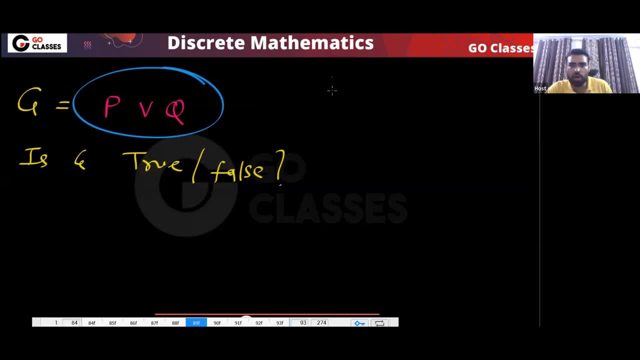 So that is the point. If you have any propositional logic expression, then to find the truth value of that expression you need the truth assignment to the variables, Correct, Yes or no, Any expression. I give you So basically what we need. 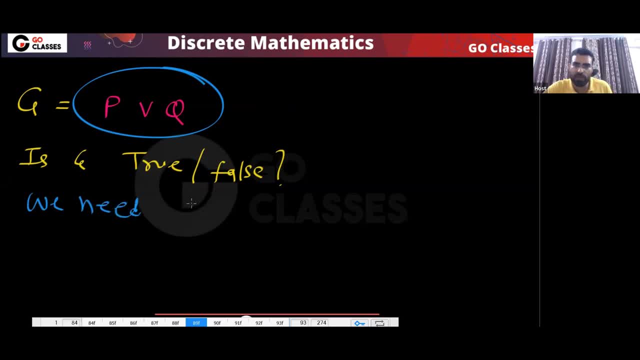 I can say what we need. We need the truth value of P, We need the truth assignment. This is what we need. We need truth assignment to P comma Q. Okay, So here, P comma Q are propositional variables. These are propositional variables. 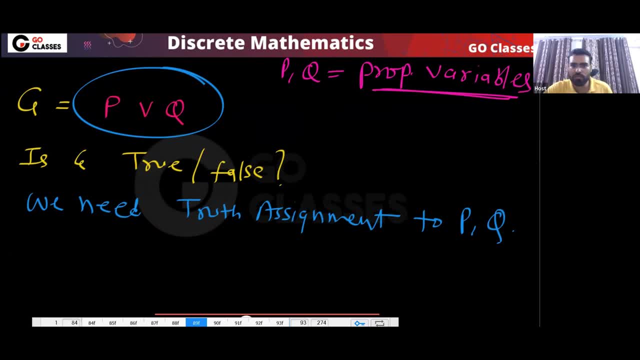 Then in this situation. So what we need, We need truth, assignment of 2 P comma Q. So this is the idea. So if you have any propositional logic expression, If you have propositional logic expression, Any propositional logic expression, 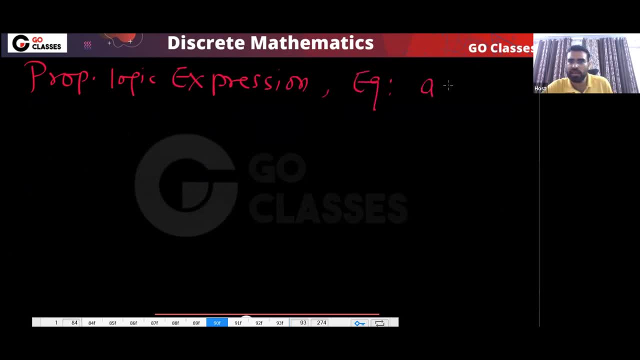 For example. if, for example, you can say like A or B, Or B implies C, Like this example, you can notice Now, in this situation, to find the truth value of this, let's assume A comma, B, comma, C, These are the propositional variable and this is your propositional expression. 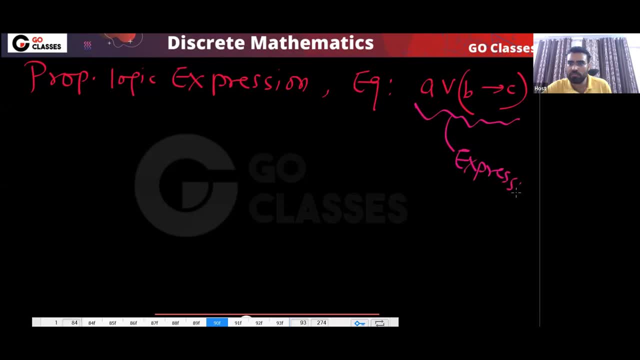 This is the expression. This is the expression. So, to find the truth value, what you need To find truth value, To find the truth value of this expression, Propositional logic expression, in short, Let me call it PLE, So to find the truth value of PLE. 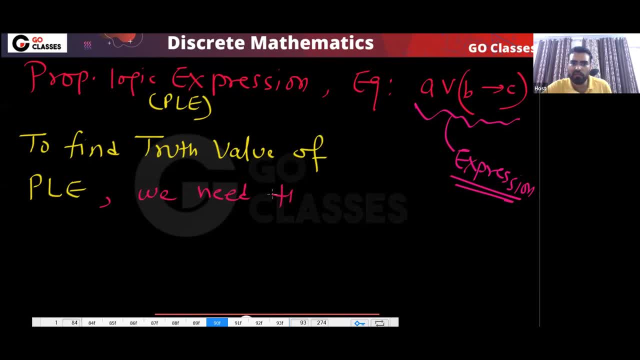 We need the truth assignment to the propositional variable. right, We need the truth assignment. What is the truth assignment to the propositional variables in that expression And this assignment? So okay, So this is the information we need. Do you need any other information? 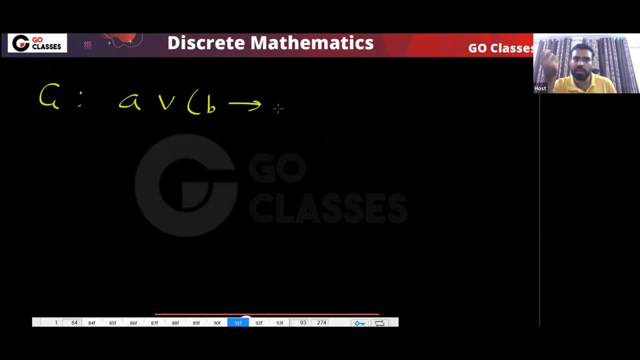 For example, if I give you this expression, let's assume A or B implies C, And this information I am giving you: that A is true, B is false, C is false. Do you need any other information? Tell me, Do you need any other information? 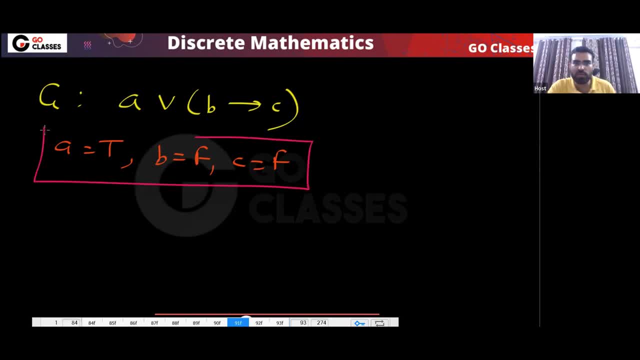 No, there is no other information you need. So this is the information you need And only this information you need. You need this information And there is no other information you need. So this is called interpretation. This is called interpretation of G. 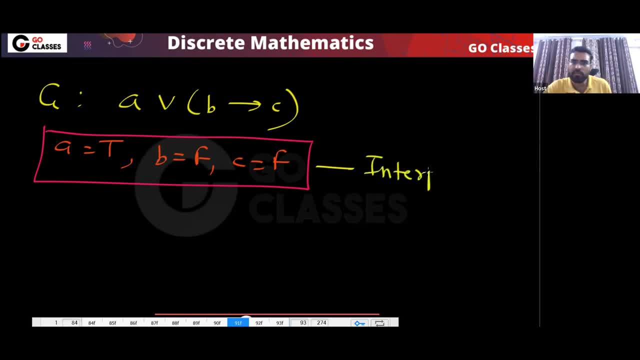 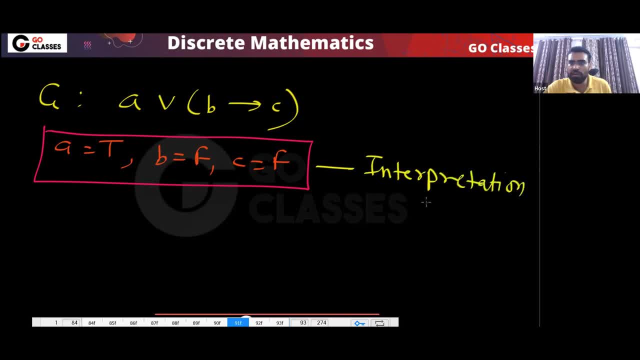 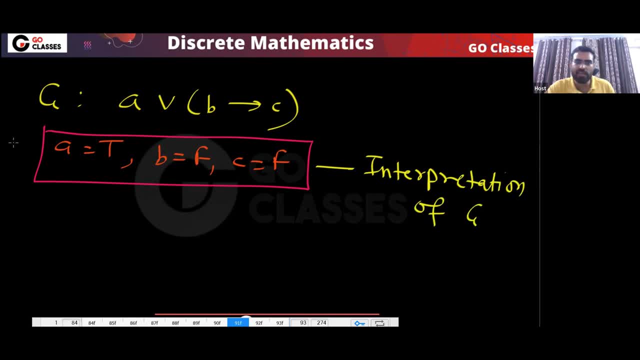 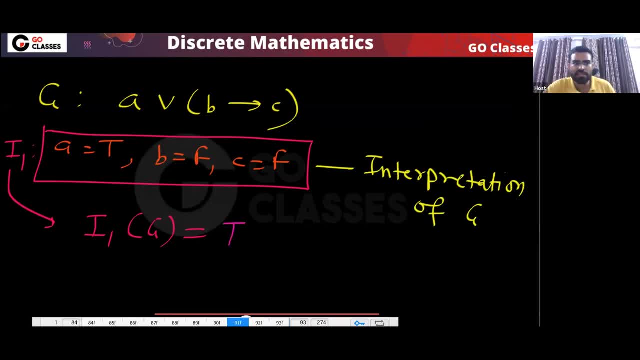 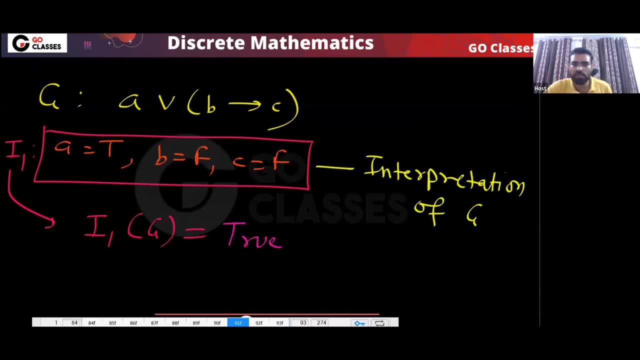 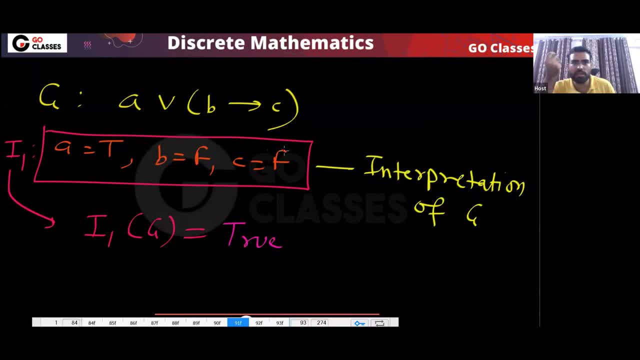 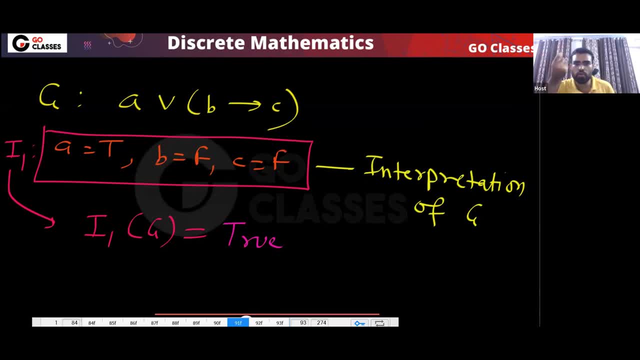 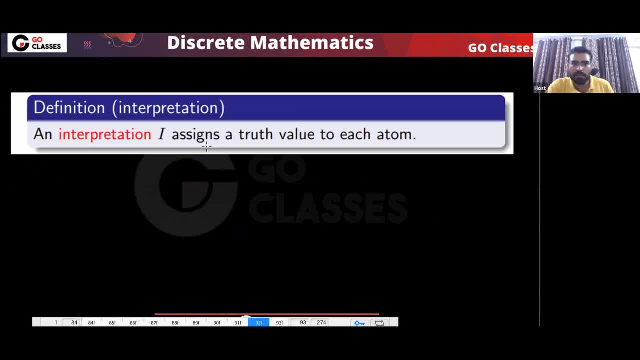 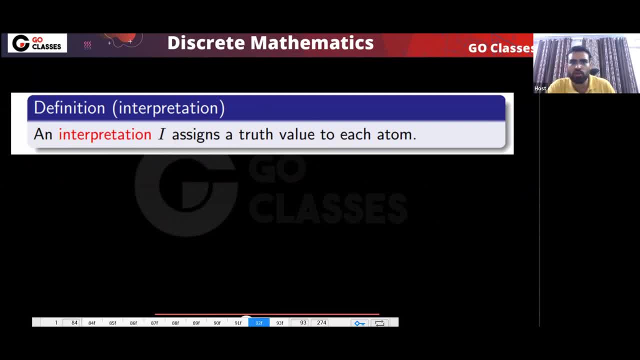 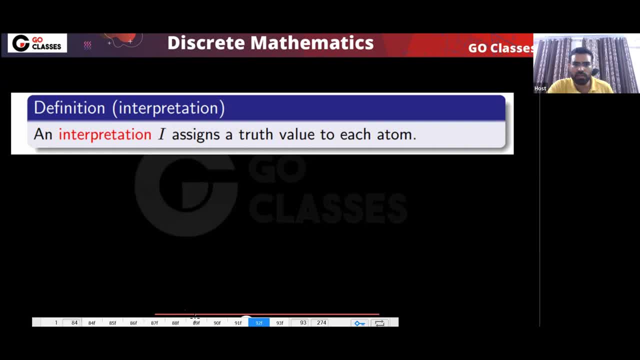 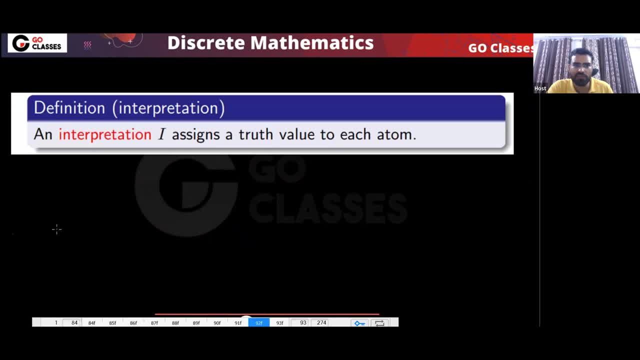 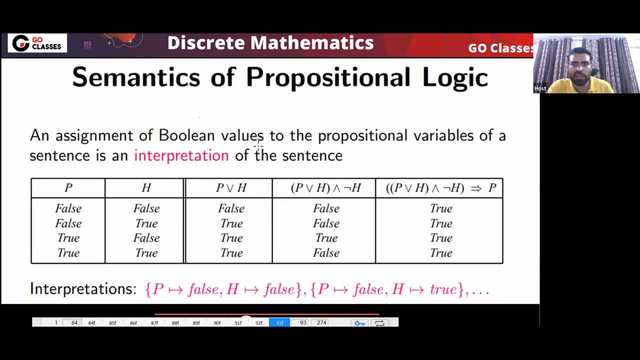 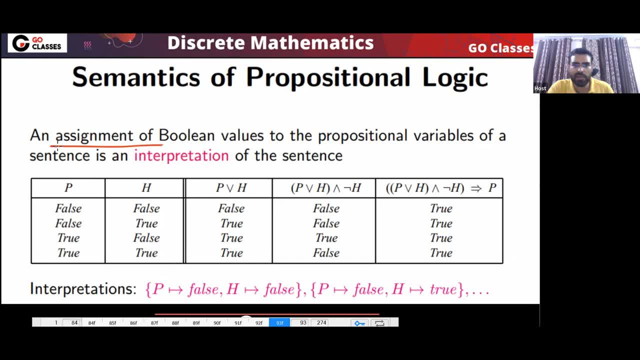 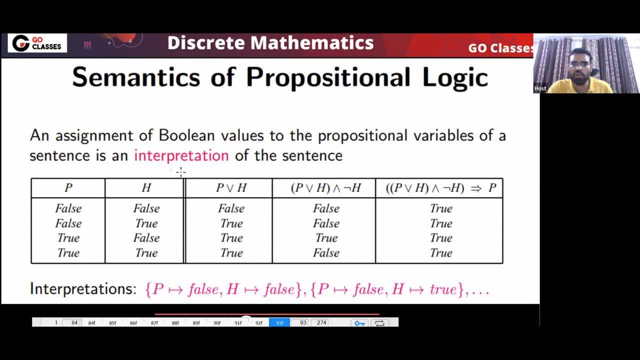 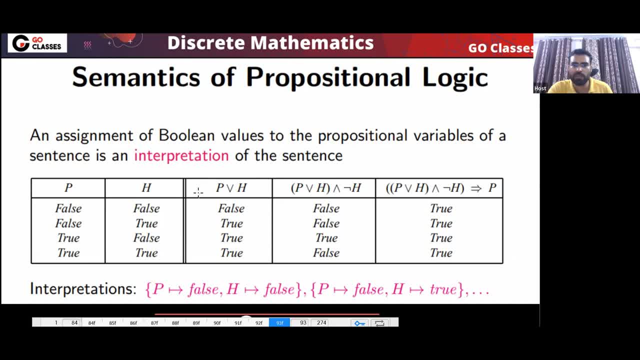 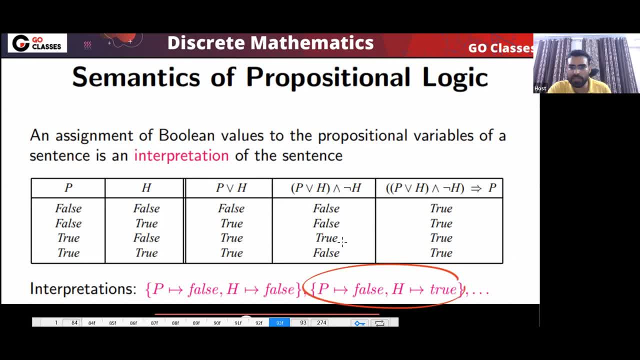 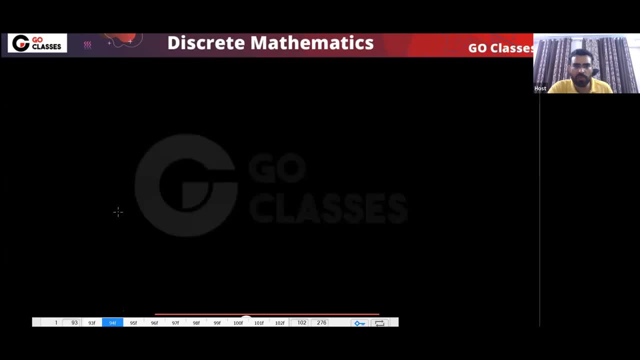 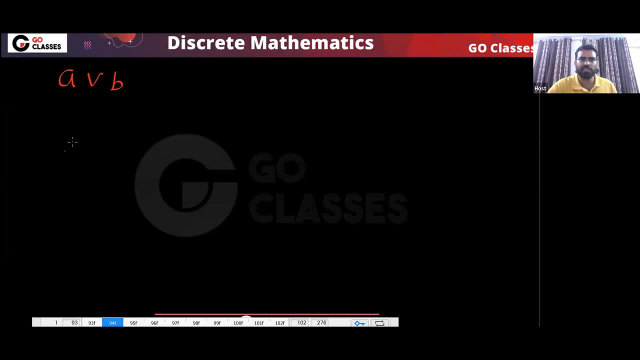 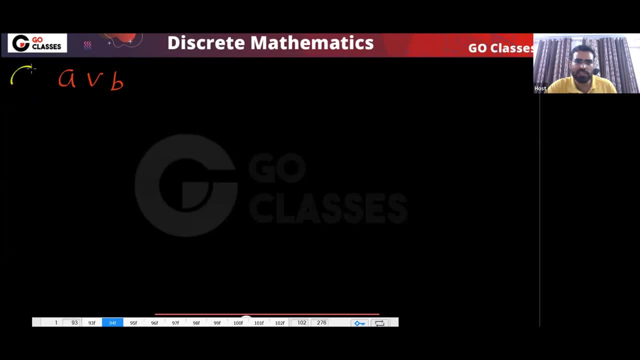 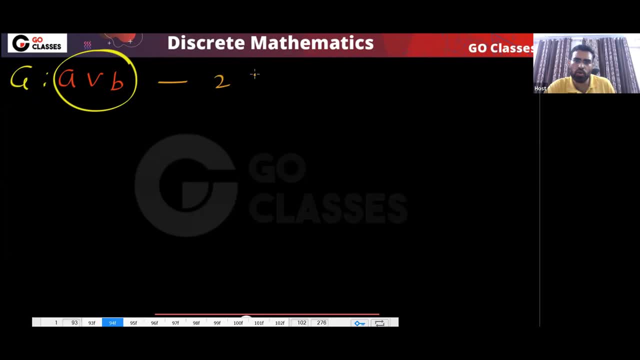 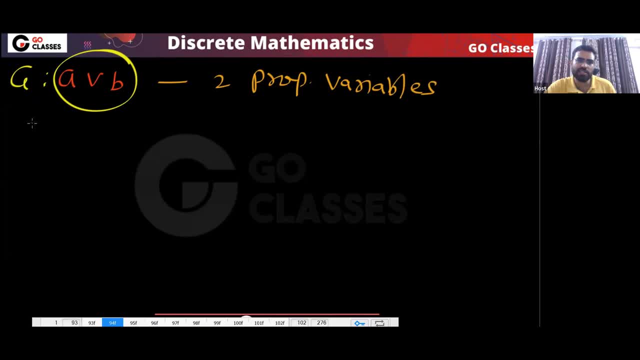 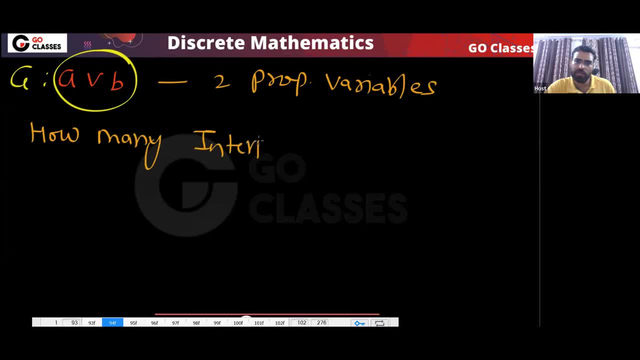 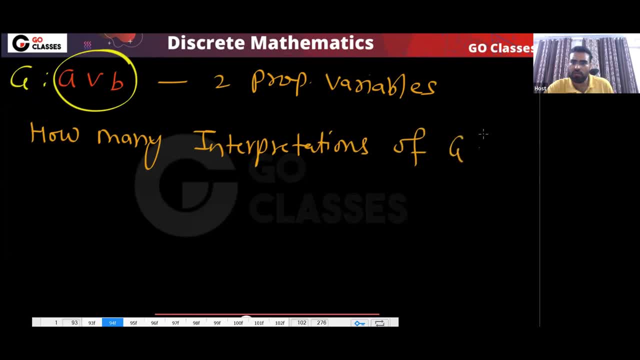 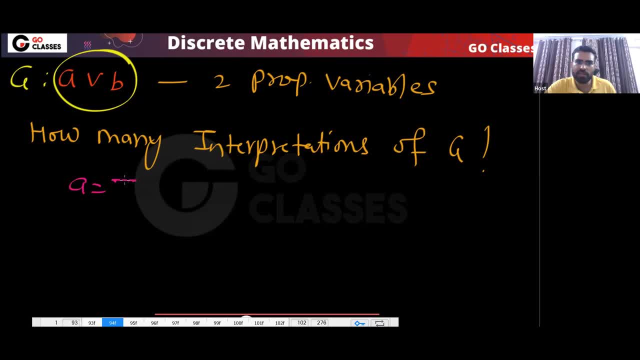 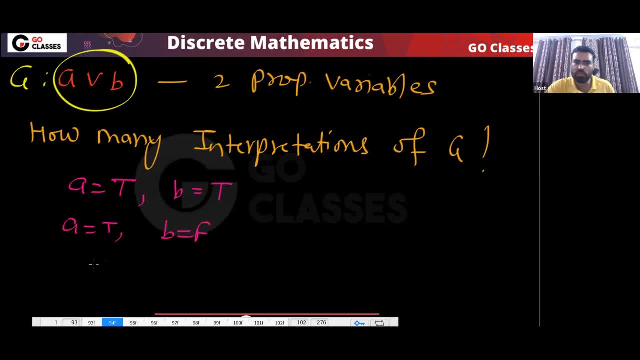 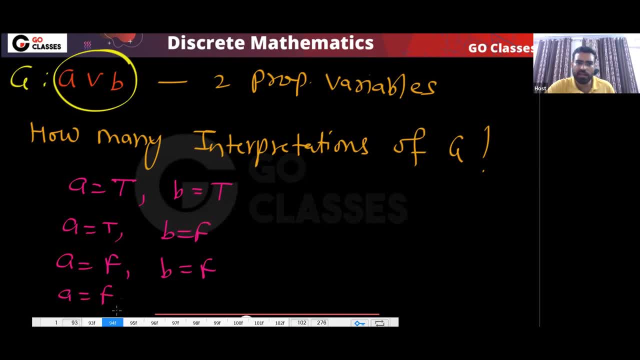 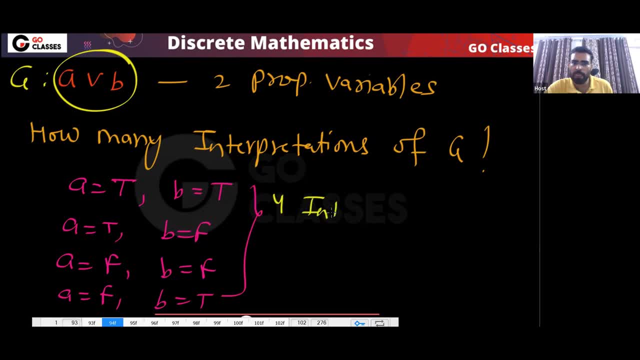 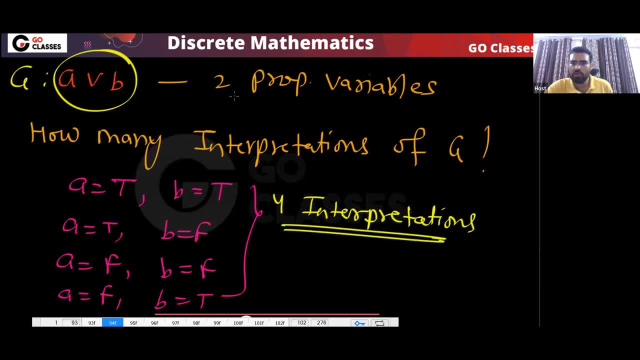 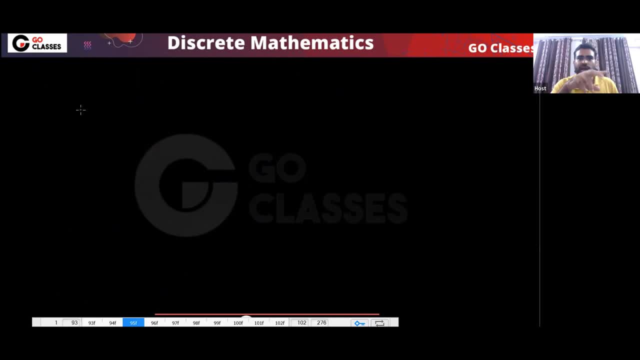 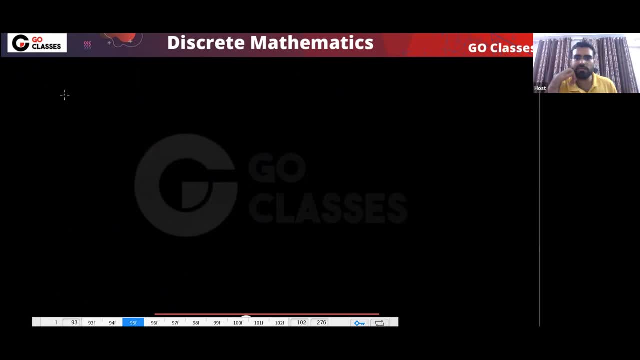 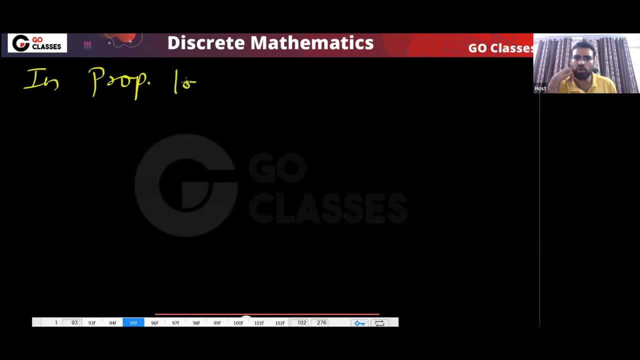 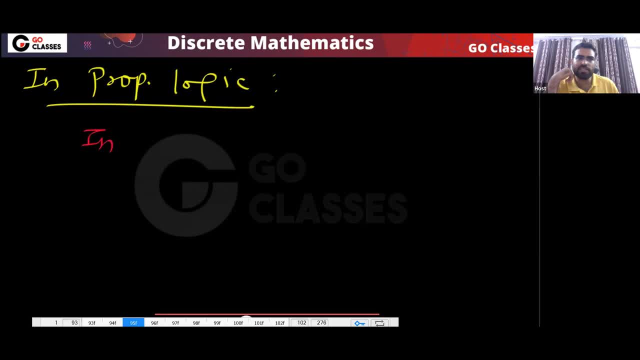 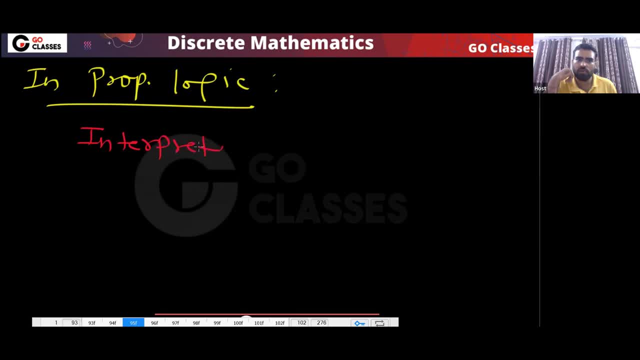 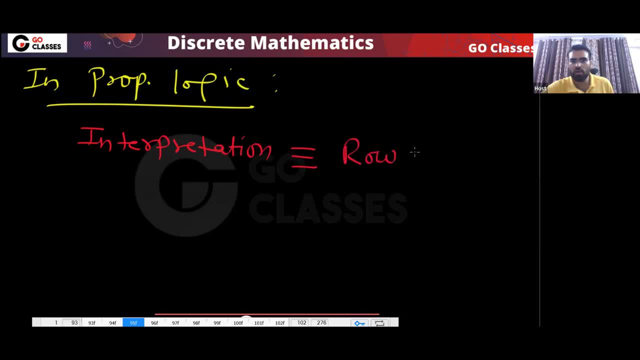 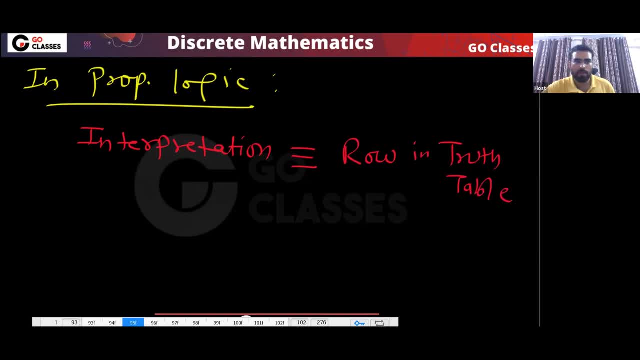 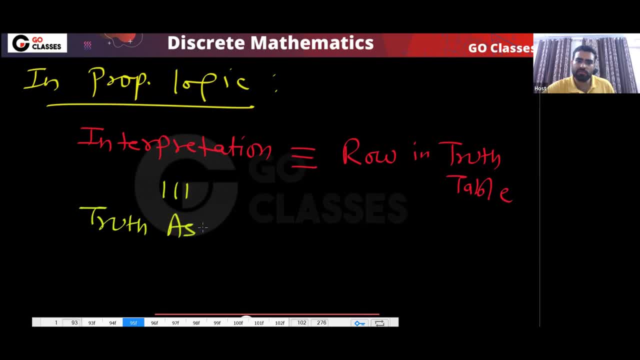 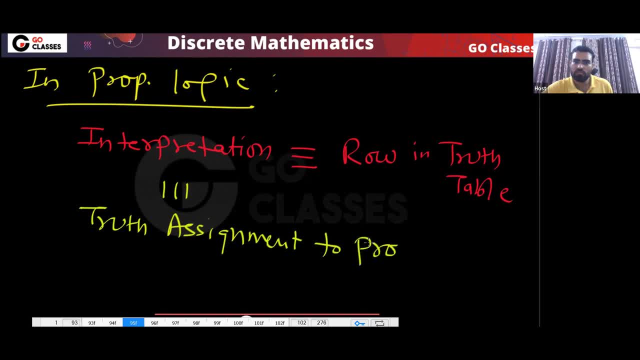 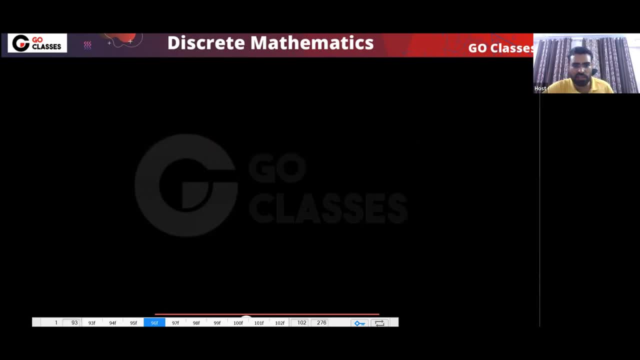 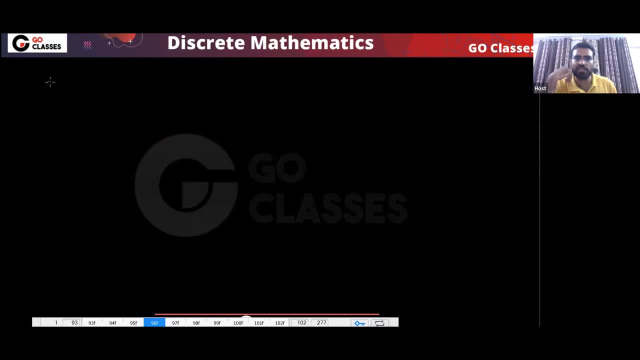 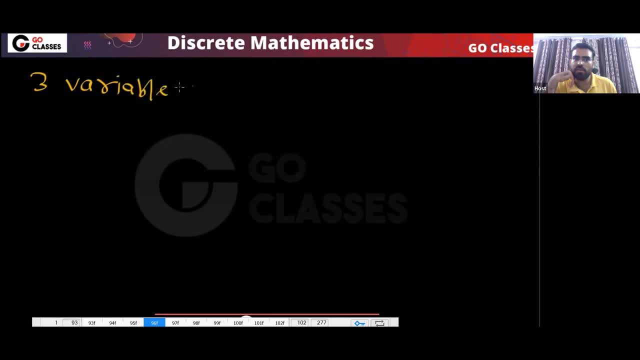 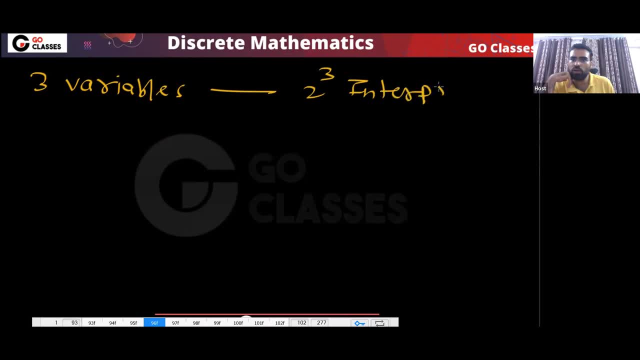 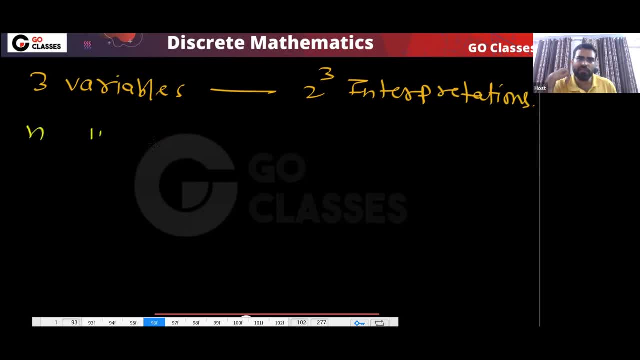 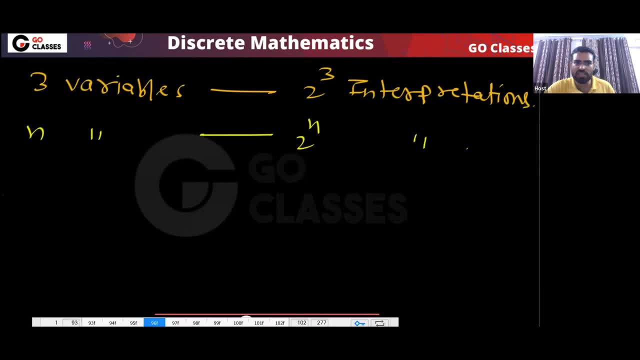 Now let me tell you some of these interpretations. for some of these interpretations, the, for example, if I give you this example, like you have this A over B, Now you can notice, means we have total four interpretations. we have. So, in short, let me write it N. 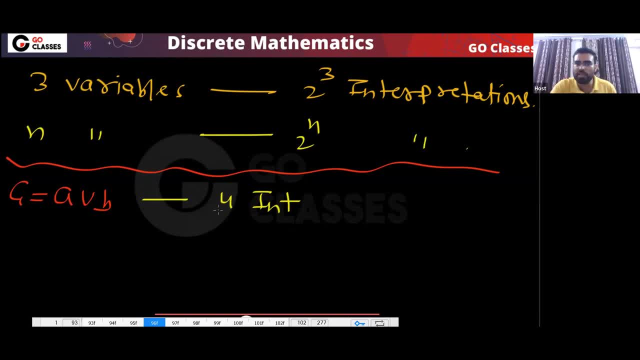 So we have total four interpretations. but how many of these interpretations this is true? for how many of these interpretations This expression is true? This expression is true only for one interpretation. So I can say only for one interpretation, sorry, only for. 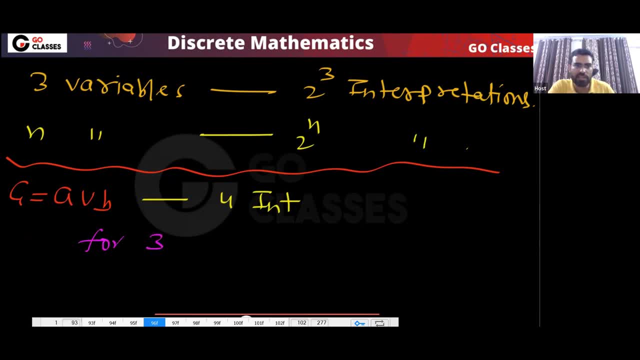 three interpretations There are. I can say there are for three interpretations. for three interpretations this G is true. So these three interpretations are known as model. We call them model. This is the definition of model. So what is a model? Model is interpretation. 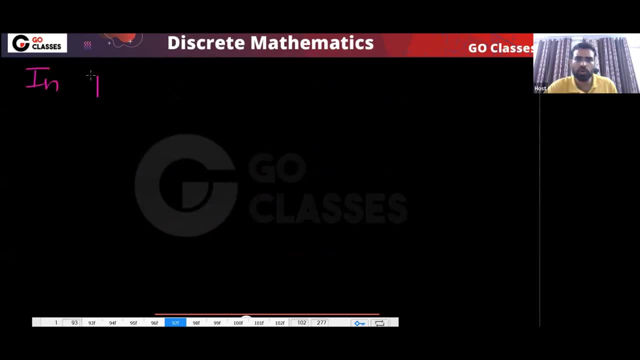 for which our expression is true. So in propositional logic- remember I'm talking about propositional logic only After some time I will discuss the first order logic. but in propositional logic, what is model? Model is an interpretation for which expression is true. 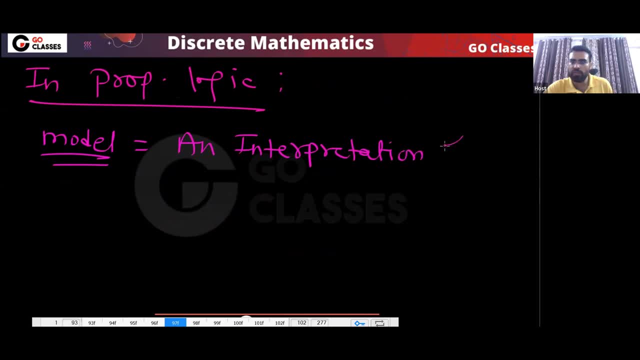 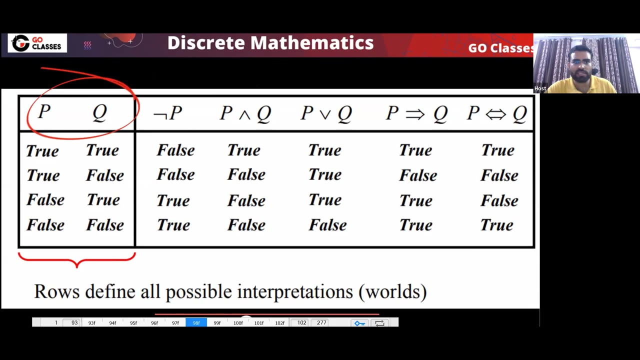 An interpretation for which expression is true. For which expression is true? Very simple, right? Yes or no, Isn't it simple? So, for example, if you have two variables, then there are four interpretations. are there So rows basically in the truth table? 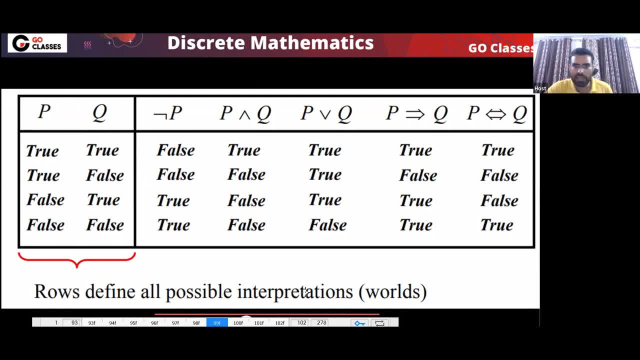 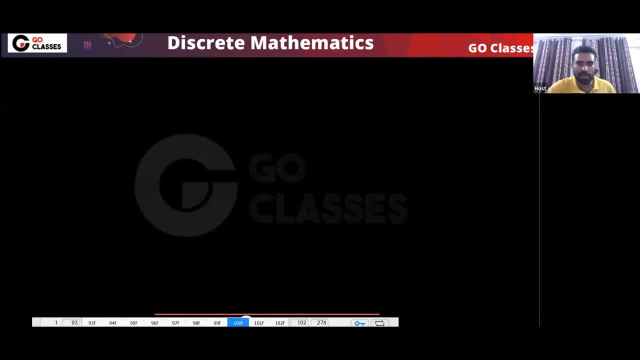 these rows are basically the interpretations. Now you tell me one thing: Interpretation is also called world. Now, how many models are there for this, For this negation P? if I ask you, for this negation P, how many models are there? This is the question. So 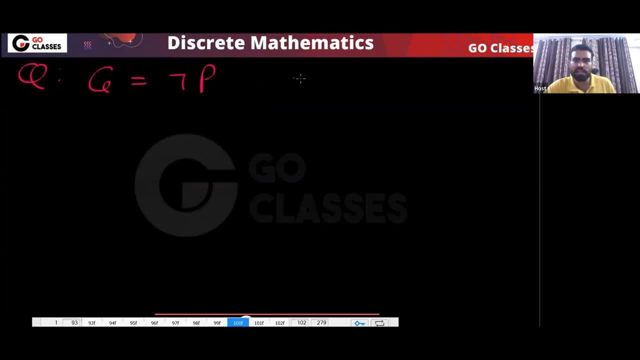 this is the expression I'm giving you: negation P: How many models are there In the simple system you have? remember, in the system you have two variables: P, Q. these two variables you have In the system. you have these two variables. My question is for this: how many models we have? 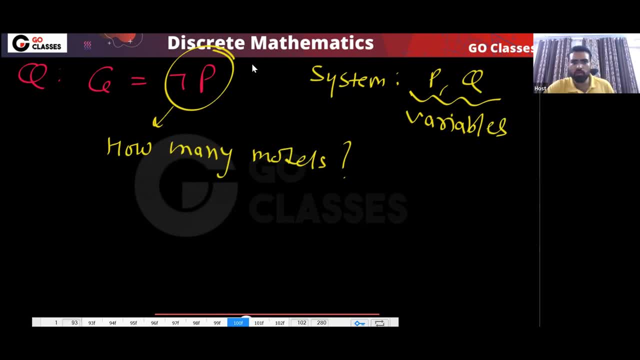 How many models we have. So here you must focus here. See: okay, in your system you have two variables. If you have two variables, you can define these two variables. See: with two variables can I define negation P Like I have P, Q? 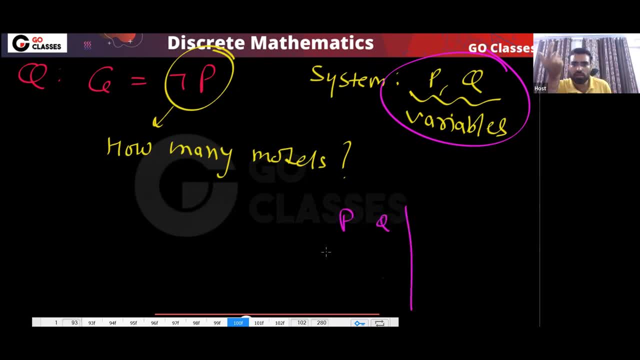 but I can define right. I don't use Q. See, it's the situation like this In my system: I have total, total, two variables. I have. Tell me, if I want to define expression, is it mandatory that I take all the variables? Tell me, is it mandatory that I take all the? 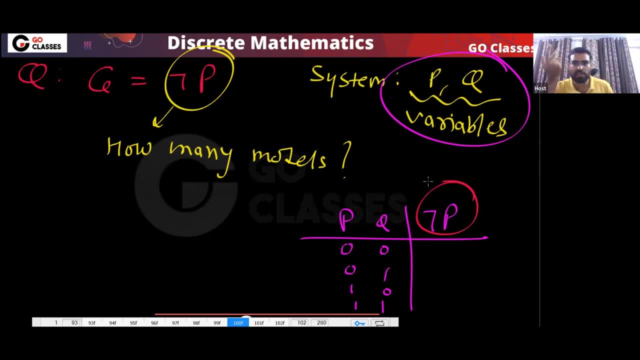 variables? No, Who told you to take all the variables? See, in the system you have these two variables, P, comma, Q. but but I can say I can define. I don't have to take all the variables. I can define negation P. what will be the negation P? that will be 1, 1, 0, 0.. So how many models? 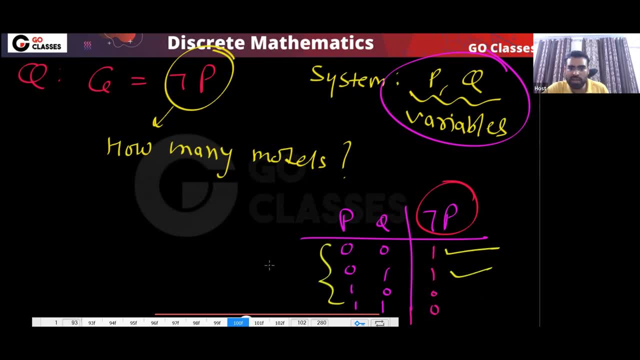 this negation P has: this is a model. This is a model. So there are total four interpretation, total four interpretation we have, and there are total two models we have. So how many models we have? number of models the question is asking. So number of models will be two. 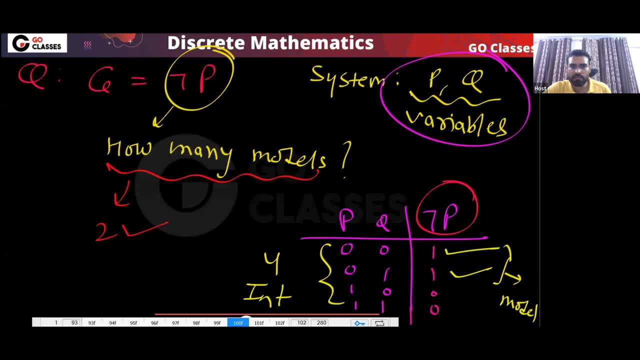 So the answer is two. Okay, It's like this. So basically, this G, this G, has two variables, but, okay, We are not using both the variables. G has two variables, but we are not using both the variables. So this is the idea. Now, if your system has only one variable, basically, 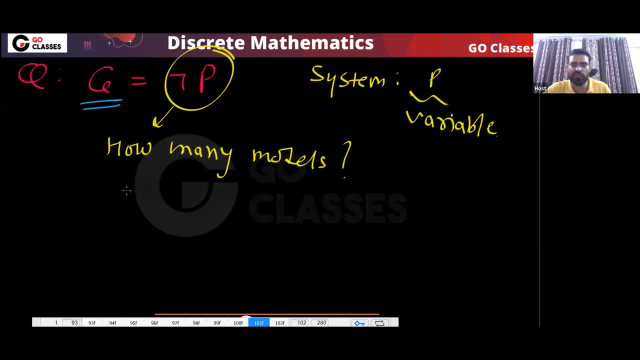 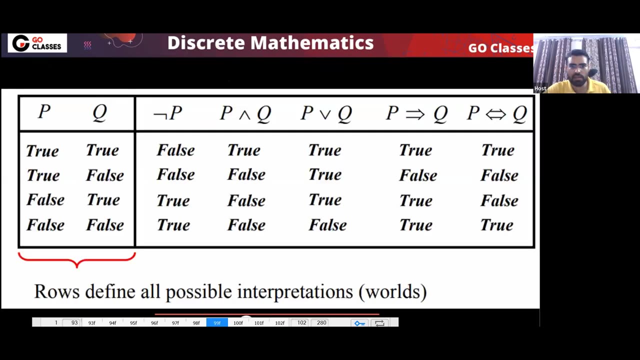 what it means. it means your G. okay, in your system, only one variable. Now, how many models are there? Now, the answer will be one. How many interpretations are there? Interpretations will be two, Interpretation is fixed, but only one model will be there. Okay, Now tell. 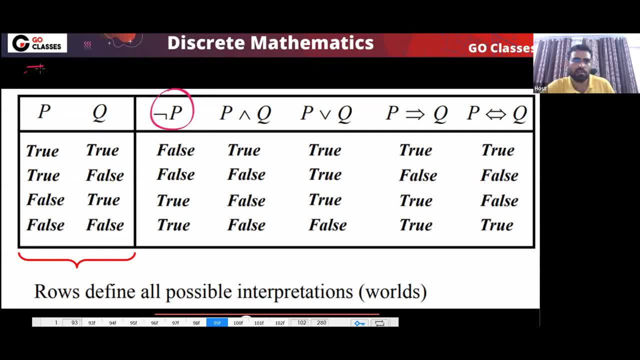 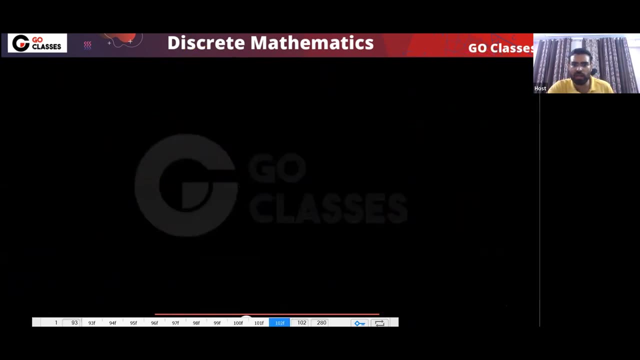 me for this: how many models you have? Number of models. Number of models. So for this you have two models. For this You have how many? Only one model. For this there are three models. For this, there are three models. For this, there are two models. Model is interpretation in which your formula 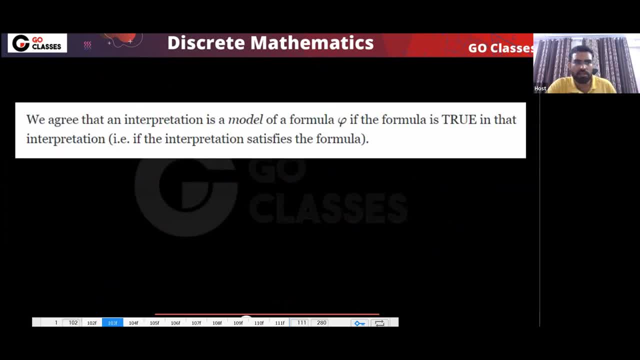 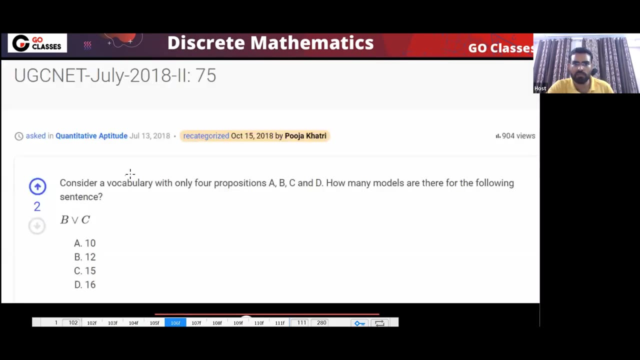 is true. So you can notice, an interpretation is model. if your formula becomes true. If your formula becomes true, then that interpretation will be called model. Means your interpretation will satisfy the formula. then this interpretation will be called model. This is a question UGC. 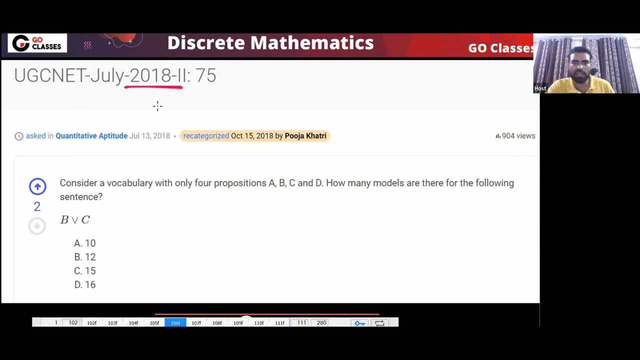 net, UGC net 2018.. So what is the answer? Tell me the answer here. So you have total four variables ABCD. How many models are there? The question is asking how many models are there for this statement. You tell me how many interpretations are there, If I ask you. so, basically, in your system. 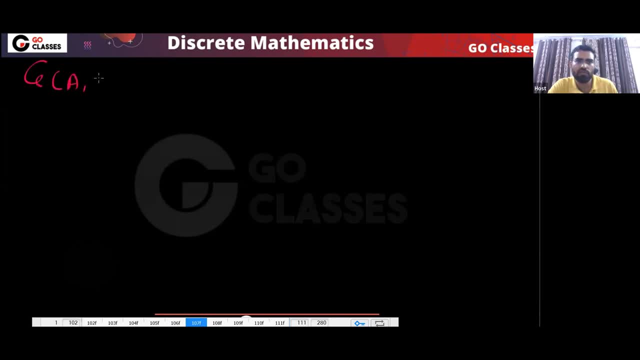 you have. it's like this. It's like this: You have total four variables, ABCD, And the formula is B or C. This is the formula. So basically, in your system you have four variables, but your expression only has two variables. How many interpretations? Tell me number of. 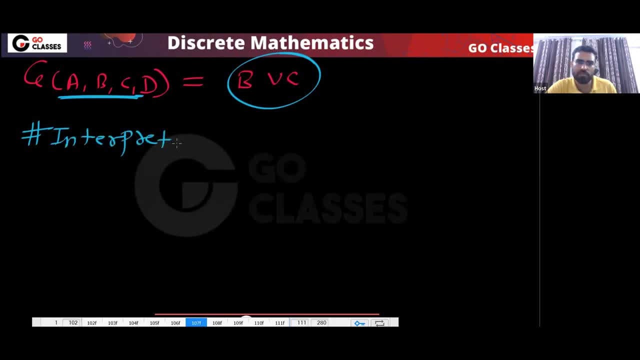 interpretations. you tell me Number of interpretations is fixed. Number of interpretations is fixed. ผmtext mechanics coloured. That is 2 power 4.. That is fixed, That will be 16.. Number of interpretations is 16.. But how many models are there? Number of models. So remember, you have total four variables. 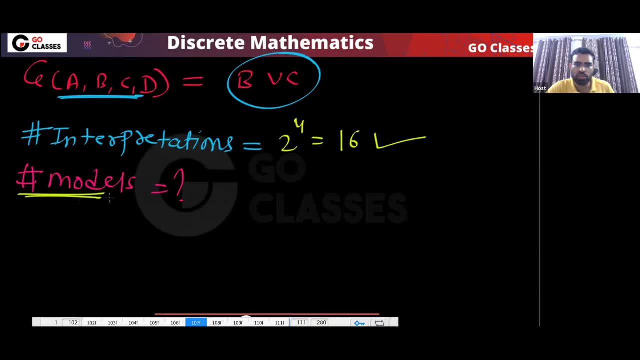 You have four variables. So model means those interpretations where B or C is true. Model basically means that B or C must be true. Okay, remember, if you want to make this true, then how many choices do you have? If you want to make this B, then how many choices? 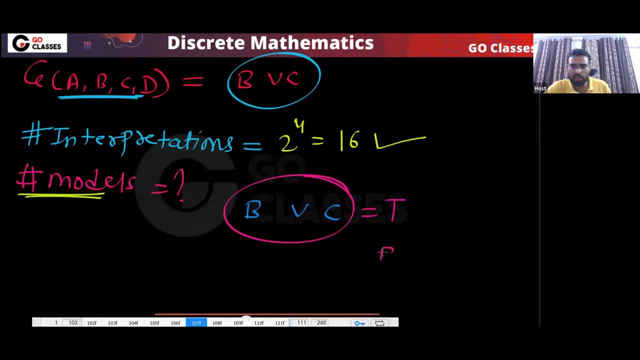 for B C. This is true, Then how many choices for B C we have? For B C, we have three choices. right For B C, we have three choices: B C together, B C together. we have three choices. 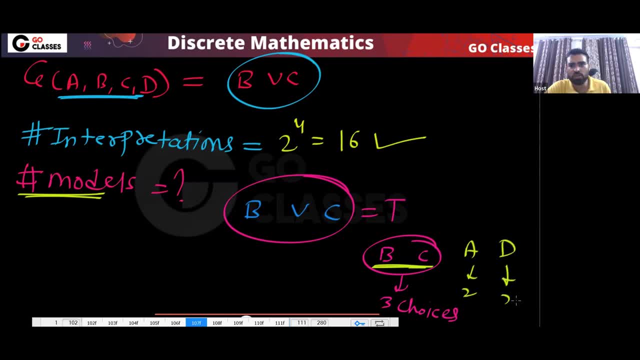 For A: how many choices? Two choices. For D: how many choices, Two choices. So the answer will be: what? 3 into 2 into 2.. Yes or no? Correct. For B, C together, we have three choices. 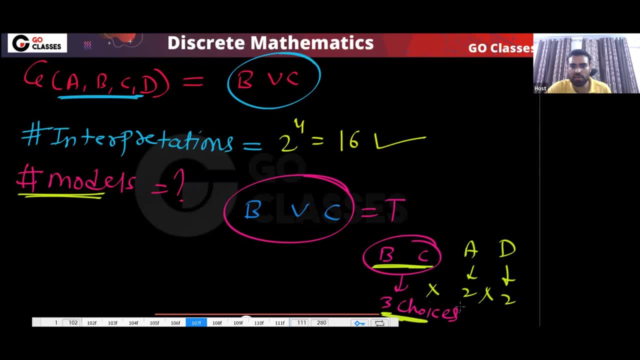 This: B, C together, they have three choices. A has two choices, D has two choices. So finally, answer will be 12.. So the number of models will be: answer will be 12.. So there will be total 12 models, But their interpretation is same, That is 16.. This is another, okay. 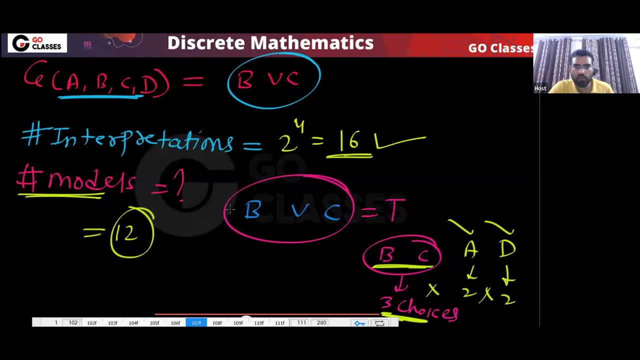 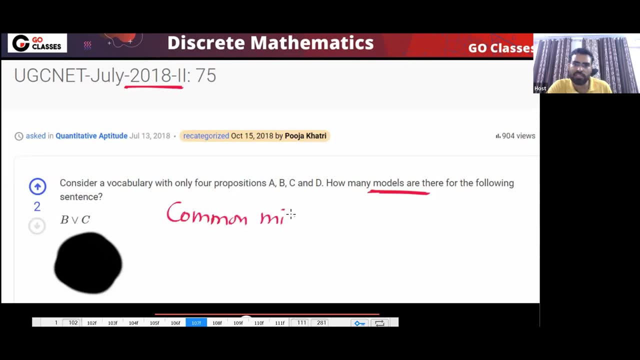 remember here one common mistake that students make. What is the common mistake? What do you think What should be the common mistake Here? the common mistake is that answer is 12.. The common mistake is that if you say answer is 3. The common mistake is answer equal to. 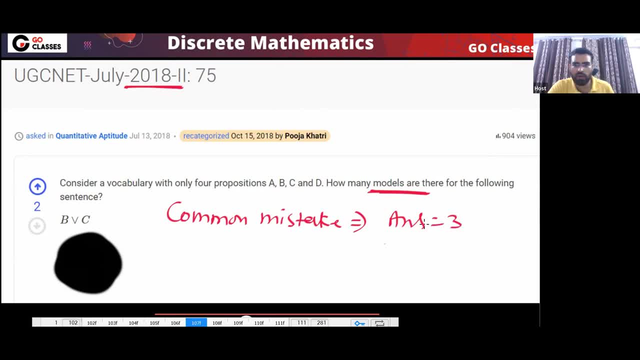 3. This is the common mistake. Why this is the common mistake? Because, remember, you will just think B or C, B or C should be true. Okay, B or C should be true. Then you will think that, okay, I have 3.. So there are three ways. So you will think that, okay, there. 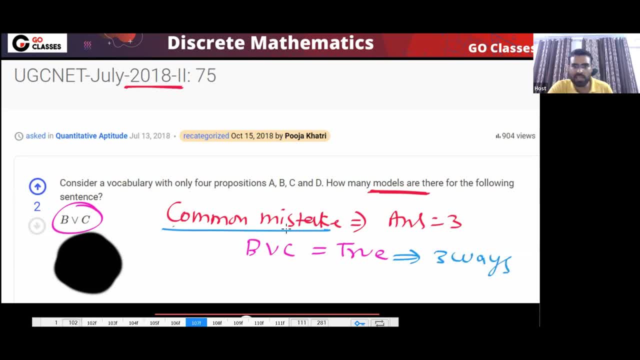 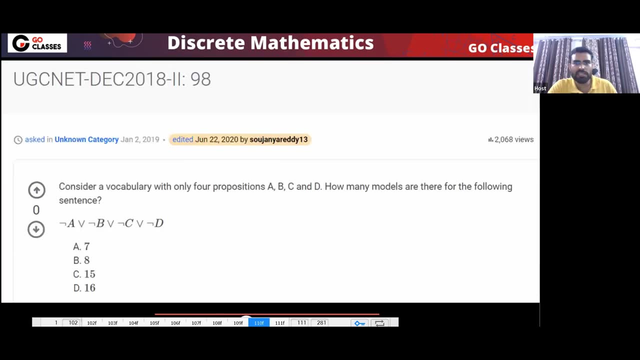 are three ways. This is the common mistake. The common mistake is ignoring. the common mistake is ignoring A D. You are ignoring A D. That is the common mistake. Okay, Now let's see this. This is another UGC net question. What is the answer? Another UGC net question. So you have total. 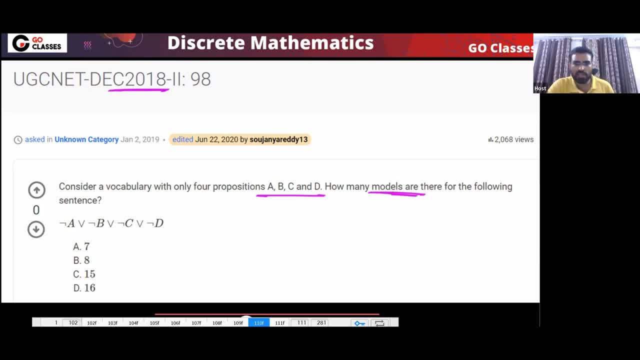 four variables. How many models? Again, the question is asking: how many models? If I ask you how many interpretations, then what is that? First, you tell me the number of models, Tell me number of interpretations. That is same right Number of interpretations. That. 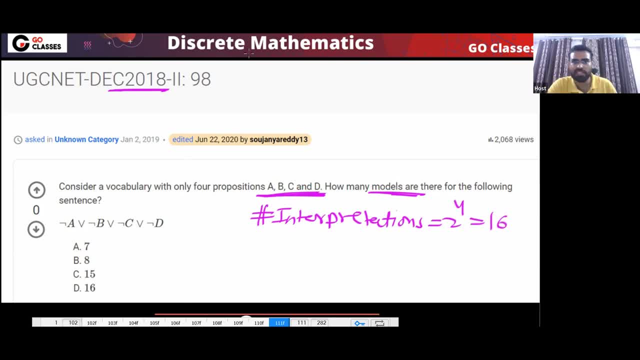 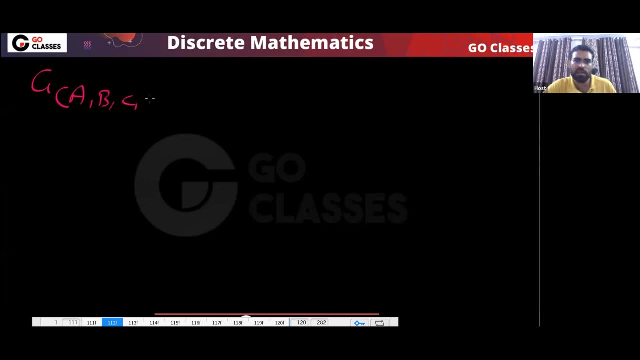 will be two power four, That is 16.. Number of interpretations will be 16.. How many models are there? How many models are there? Basically, this would be true. Remember, basically, your expression is like this: In your system you have total, four variables And your expression: is negation A over negation B over B over B In the final answer, you are left with a suicidal answer. Then what is the answer? You are simultaneously calling anyone non- GOD. So you go front-pass to the conclusion. You go from À to spirit. A should go forward Here. 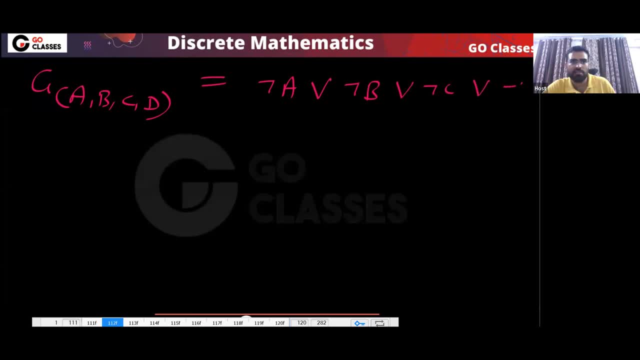 or negation C or negation D? Okay, tell me when it will become false Instead of writing. okay, instead of finding modal, you can find co-modal. Remember what is co-modal? Let me tell you. Let me tell you what is co-modal. What do you think? What? 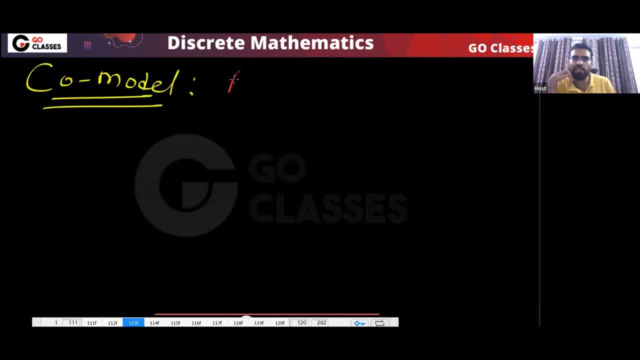 is the definition of co-modal. Co-modal means an interpretation for which formula is false, This is called co-modal. And interpretation for which formula is false, for which expression is false, This is called co-modal. So here, how many LOords will be there, If you want? 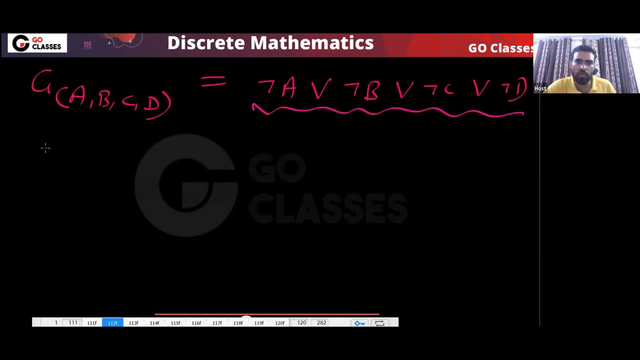 to make it false. there is only one way, right, See how many co-modals. So so just find the number of co-models. the simply find the number of co-models. number of models will be one, because if you want to make it false, if you want to make this complete, 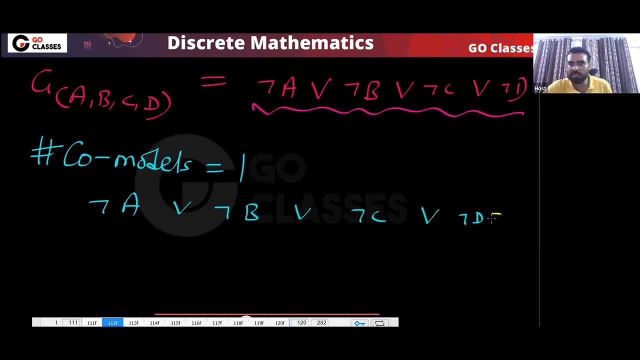 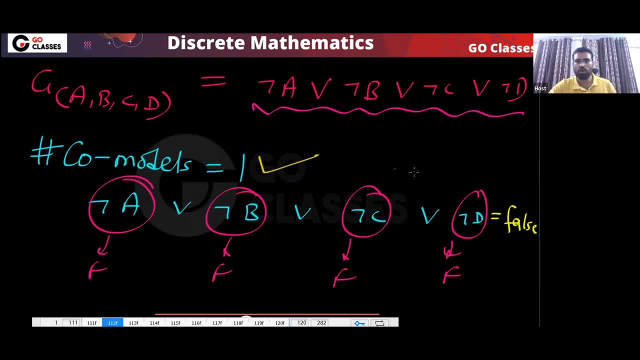 true. So I can say: number of core model is only one, So number of models is a total 15. in this situation, If number of core model is one, then number of model will be total 15.. So I can say: number of core models, what number of models? what is that? That is it. 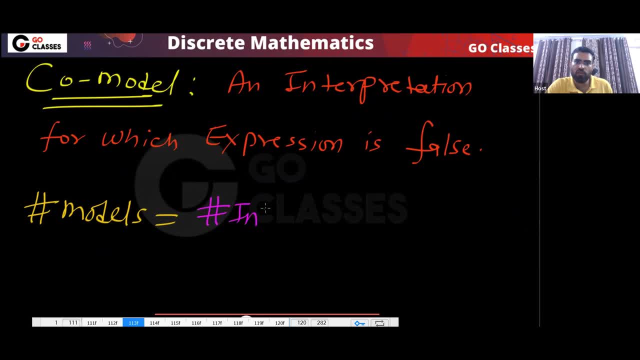 What is the formula? Number of models is equal to number of interpretations minus number of core models. Right, See here What I'm saying. if you take this, for example, if you take this expression like, let's assume you have this expression, a, comma, B, and your expression is negation, A implies B. Now in 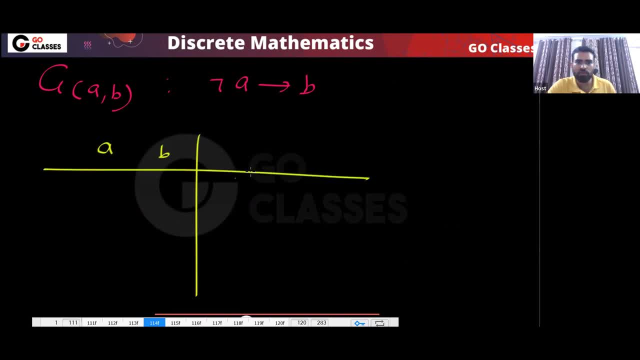 this situation. you have total, two variables. Total, how many variables? you have Two variables, Okay, 0 0 0, 1, 1 0, 1, 1.. And this is your formula G. So what will be the truth? value The truth. 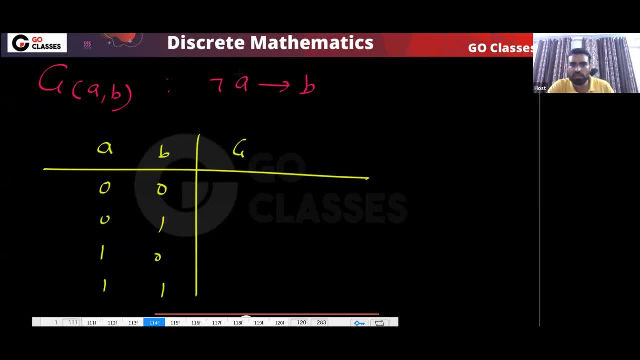 table what that will be, So you can notice that it will be false only when this is true, Means when A is false and B is false. When A is false and B is false In this situation, this will be false In all other situations. Now let me tell you. 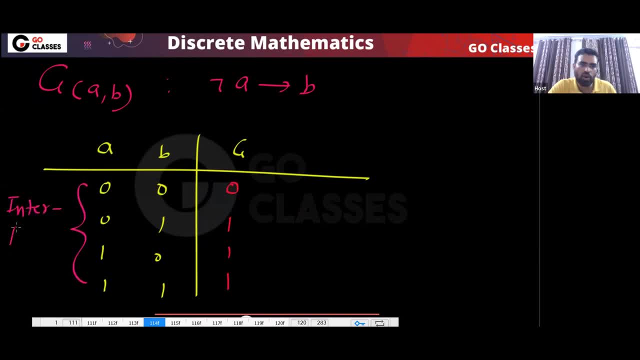 all these are called interpretations. See, all of them are interpretations. All of them are interpretations. So how many interpretations Total four interpretations. This interpretation is called co-modal. This interpretation is co-modal. This is called co-modal. This interpretation is called co-modal. 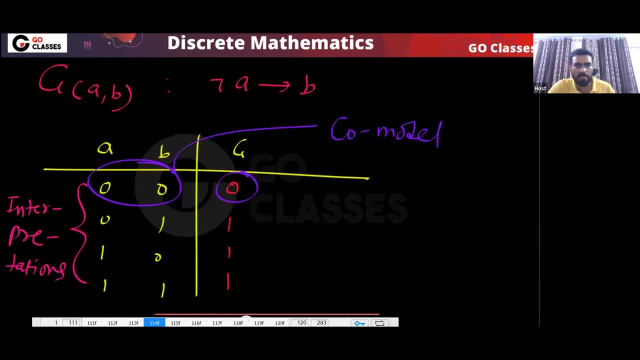 Because here you have false And this interpretation, these interpretations are called modal, These interpretations are called modal. Is it clear now The definition of modal, co-modal, is it clear now? Let's take just another example. Let's assume you have a formula And this: 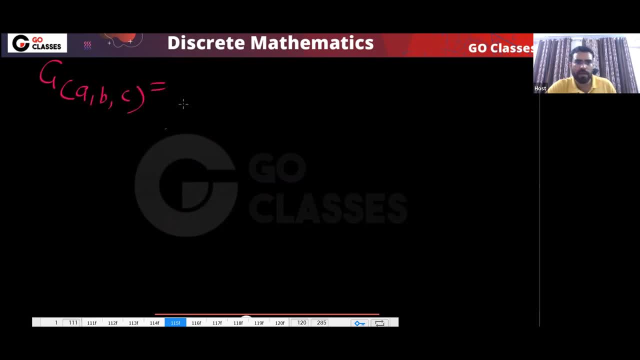 is like you have total three variables And so let's assume you have a formula. Let's assume you have three variables And the formula is A bar. Now tell me how many modals are there, How many co-models and how many interpretations? Now, in this situation, you 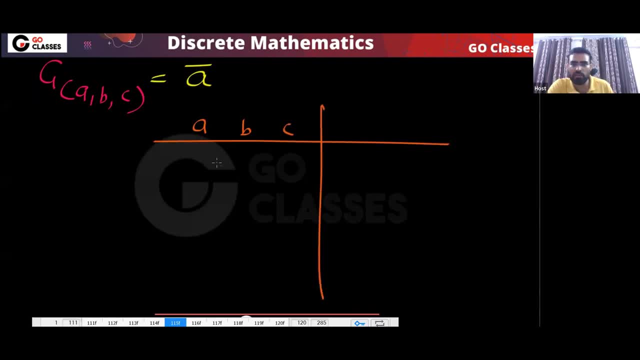 have total three variables: A, B, C. Remember: total three variables you have. Okay, so you have total three variables. So how many interpretations will be there? There will be total four interpretations. Okay So, Okay So. 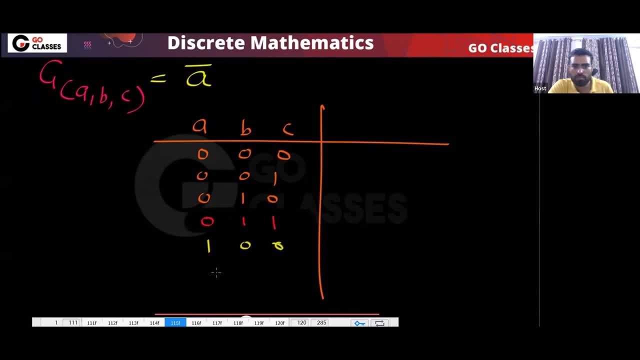 And this is your formula: negation of A, negation of A, That will be 1, 1, 1, 1, 0, 0, 0, 0.. Now let me tell you that all these are called interpretations. all of them are interpretations. 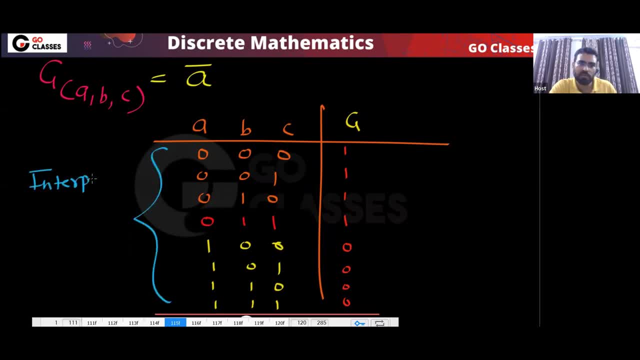 Okay, all of them, these are interpretations. So how many interpretations we have? Total, eight interpretations we have. All of them are interpretations. These are called, remember, yes or no? these are your. I can say here, you can notice here. 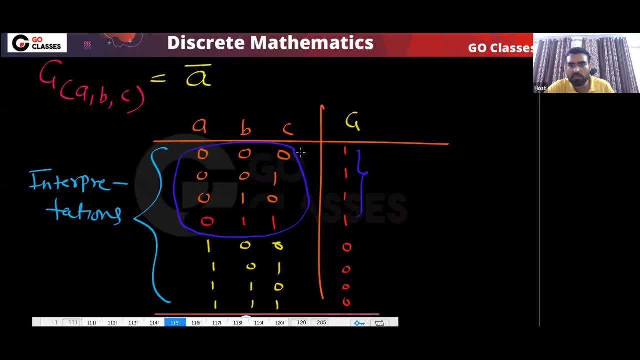 G is true. So these are your models. These are the models, because here your expression is true And these are co-models. And what can you say? You can say that these are co-models, These interpretations are co-models. 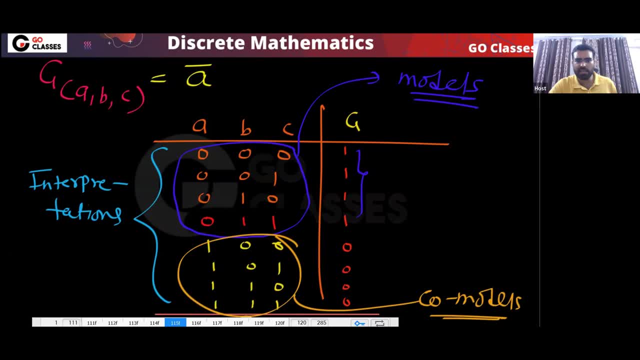 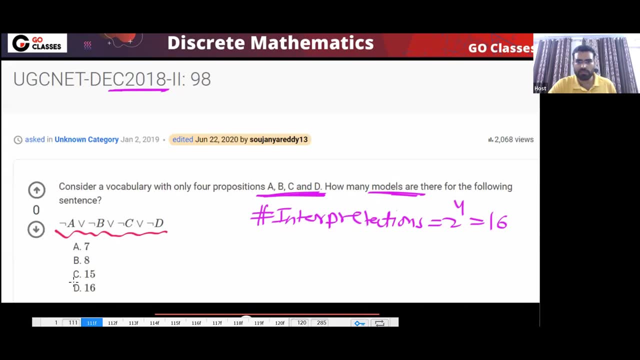 Anyone has any doubt right now? still, do you have any doubt? So the answer will be here. the answer will be 15.. So number of models- here you can notice, number of models will be 15.. Number of co-models will be only 1.. 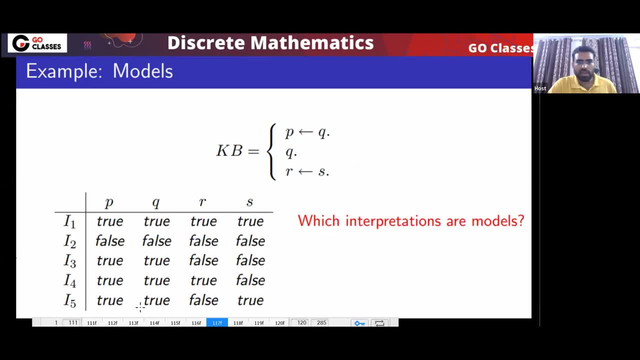 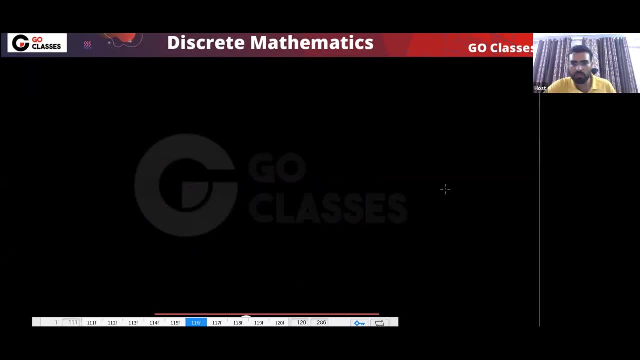 Now. so here you can notice sometimes. let me tell you one more thing- that if a complete set of formula is given to you, If a complete set of formula is given to you, then for that formula- like, for example, if I give you a complete set, let me okay. 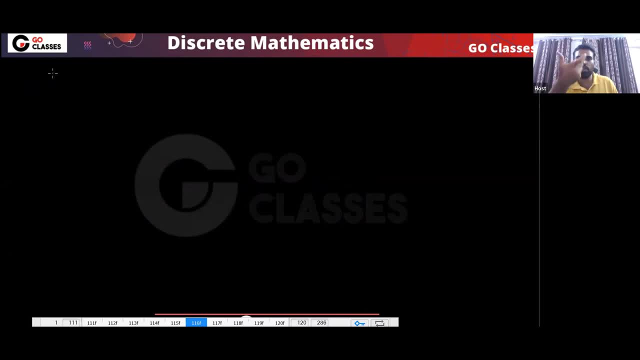 So let's assume I give you a complete set like this is called knowledge base, I told you right. So if I give you a complete set of formulas, so let's assume you have a set of expressions, set of propositional logic expressions. 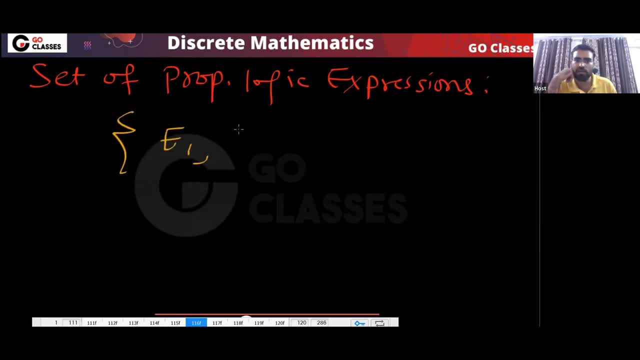 So you have set of propositional logic expressions Like okay, E1, E2 and so on, e, n. Then tell me what will be the model for this? For this, what will be the model? Let me call it Kb. 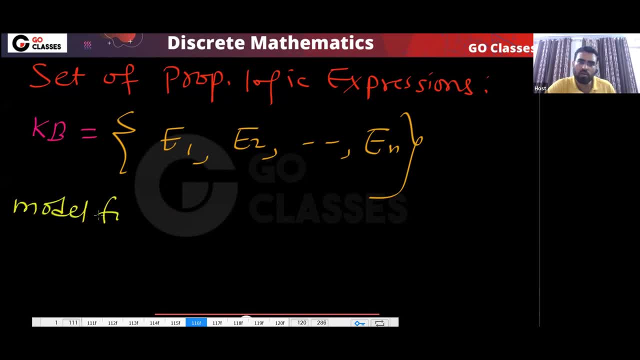 Now, what is the model for Kb, What that means Model for Kb, What that means? That means all of them should become true right When all are becoming true right. So I can say basically, those interpretations spare for which I can say those interpretations. 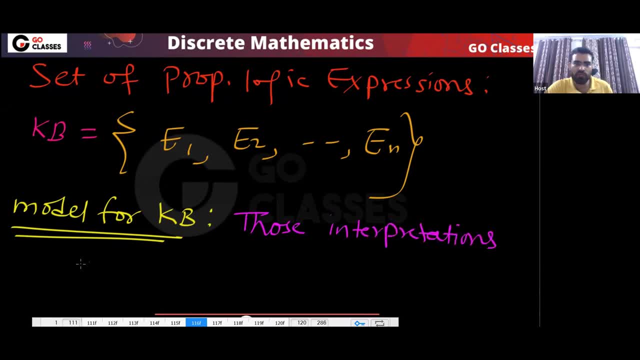 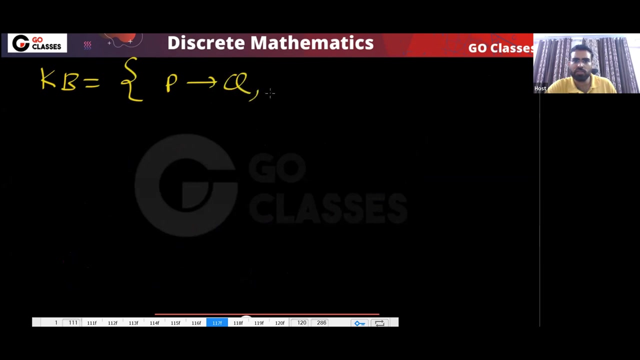 those interpretations for which all the formulas become true, for which all the expressions become true. So, for example, if I give you- let's assume I give you- this is the set of formula- I give you- P implies Q comma, Q comma R, then tell me how many interpretations are there. 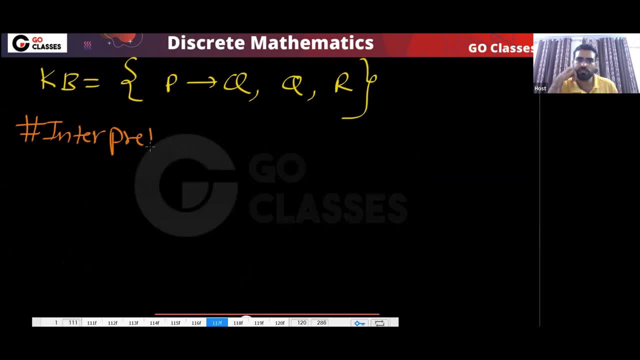 First you tell me the number of interpretations. Number of interpretation is defined, is decided by how many variables you have. So total three variables you have. so that will be two power three and that will be your eight. So basically that is two power number of variables. number of propositional variables. 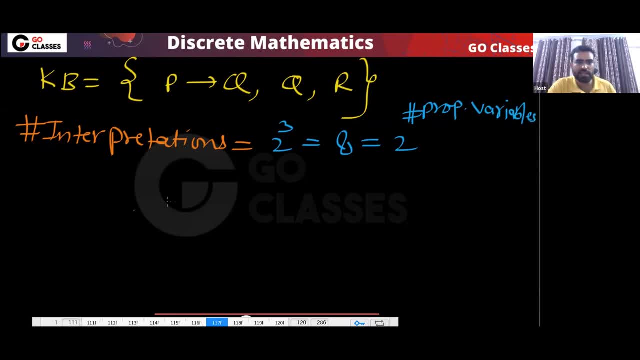 So this is very clear. note: this is very simple. so total interpretations: are there eight? how many models are there? how many models are there? remember, model means how many models are there. model basically means that all of them should become true. if you want model, then what it means: how many? 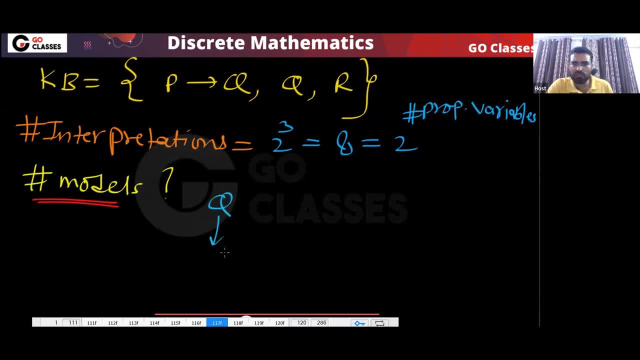 choices for q. tell me how many choices for q? only one, because q must be true. i am finding model okay. model basically means that okay, what is model? model is an interpretation where all of them are becoming true, so i can say that this also should be true. this also should. 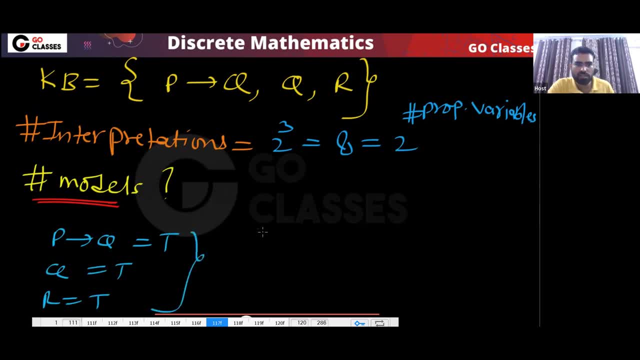 be true and this also should be true. now you can notice that for q, only one choice i have. for this q, only one choice i have. for r, only one choice i have. but for p, how many choices i have. for p, i have two choices right. so for p, i have two choices, correct. so for q there is no choice, because 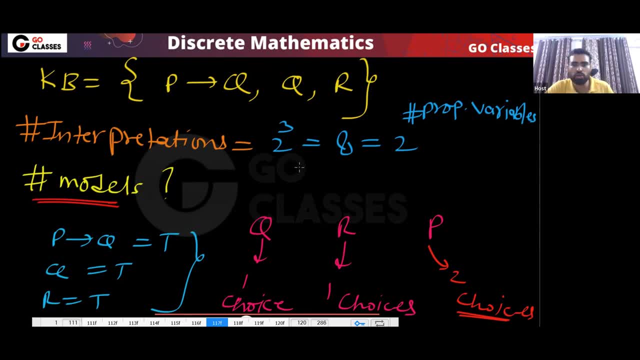 q must be true, r must be true, but for p i have two choices. so how many models? i have two and how many co-models? automatically number of co-models will be six, because number of co-model means number of interpretation minus number of models. so that will be six. another: 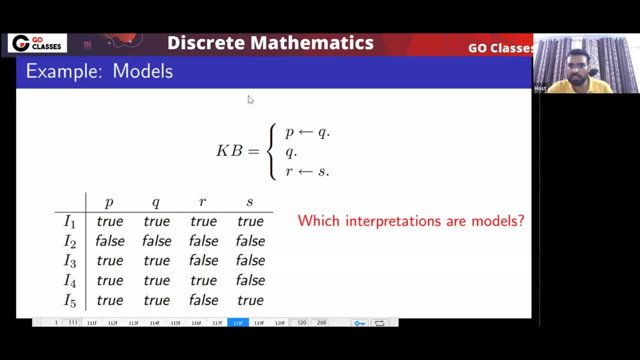 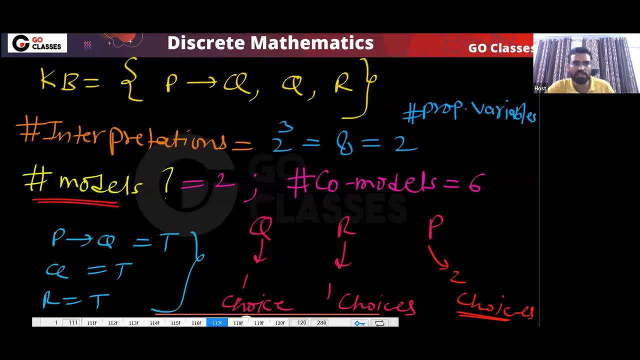 example this: which of these interpretation is model allah? this is the system. look at the system, see allah. we have three formula: this formula, this formula, this formula i want model. model means all the formula must be true, right, all the formula must be true. this q must be true, this r must be true and this must be true. 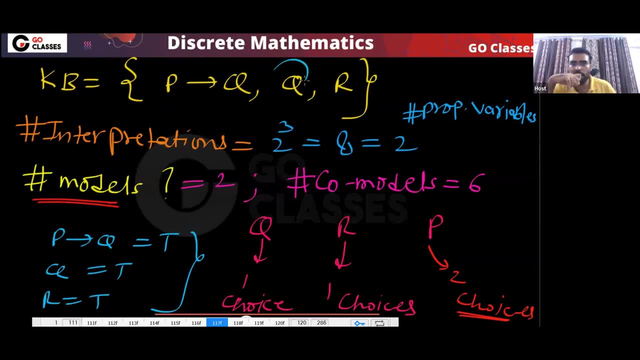 every formula must be true, right, yes or no? this is a formula, this must be true. this is a formula. this must be true. this is a formula, this must be true. so for q there is only one choice, because q must be true. so q has to be true. q definitely has to be true. okay, tell. 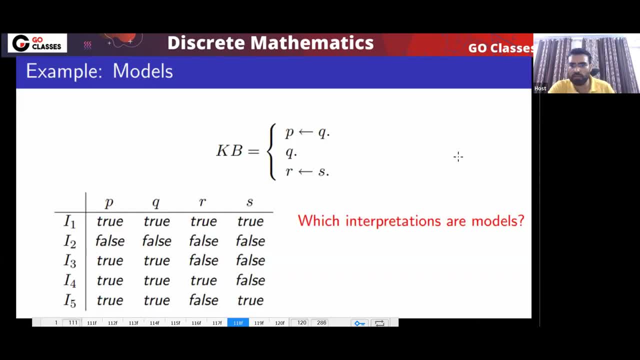 me about here. which of these interpretation is model? so which of them is model? which interpretation is model? for this? so definitely you can notice whatever, whatever interpretation you take as a model, then q must be true. so q must be true. now, this is all of the models, that is. 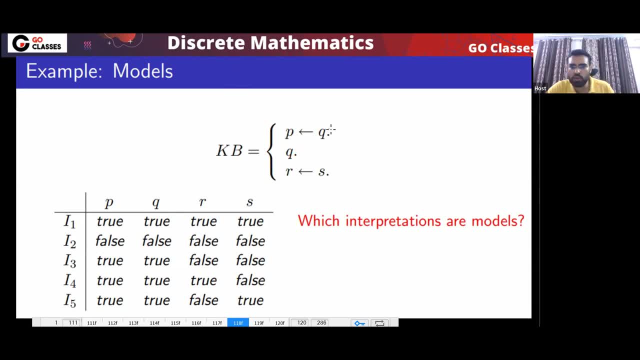 But Q must be true, right, Q must be true. And if Q is true, then what should happen? tell me. If Q is true, then definitely P must be true, right? So Q must be true, automatically, P also must be true. 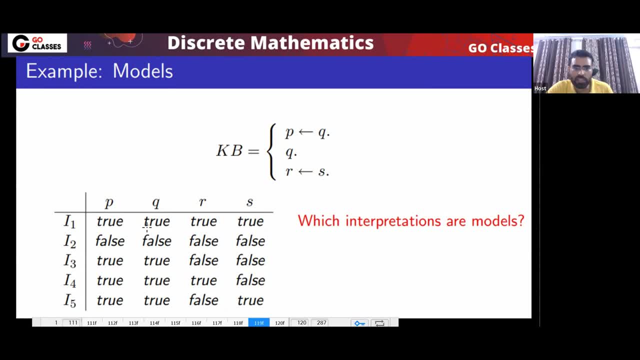 So I can say which of them is model. you can just check it out. See: Q must be true. See here: Q is false. So this is definitely not a model. Because Q is false, so this is definitely not model. This interpretation is definitely not model. 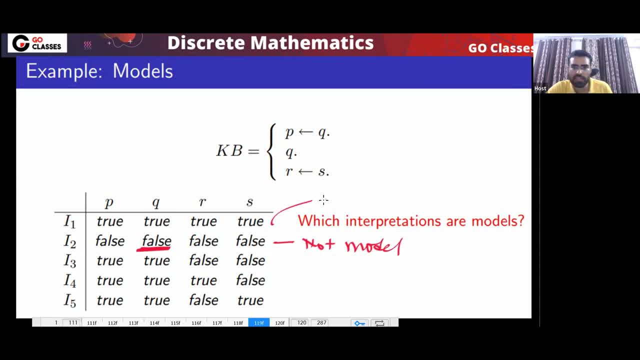 And you can notice all are true. So, yes, this is a model. I can say this is definitely a model. Remember one thing: Q must be true, And if Q is true, then P must be true, because Q implies P. This is Q implies P. Remember: 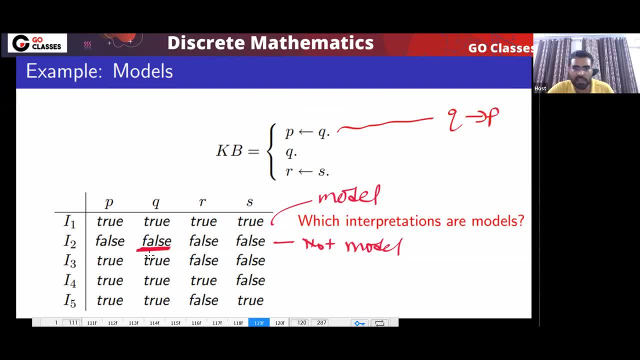 this is: Q implies P. So here I can say: Q must be true And P also must be true, P also must be true. And then you have S implies R. This means S implies R. So S implies R. So here. 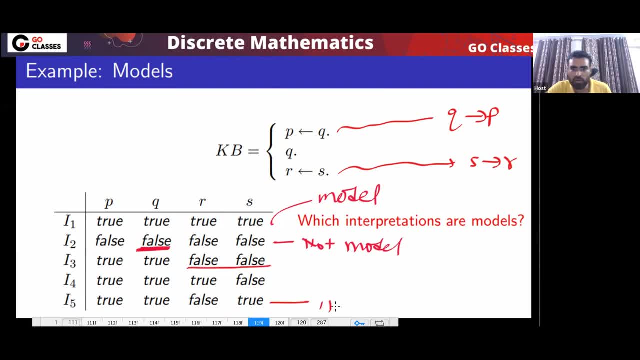 Both are okay. S implies R, So I can say: this is not model, This interpretation is not model. everything else is a model. So I can say: this and this, these are models. Is it clear? So the answer will be this: 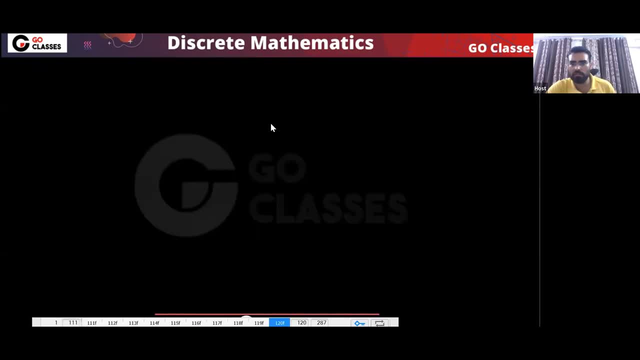 How many models are there total? How many models are there total? So, for this knowledge base, how many models are there total? Number of models? total number of models. Remember number of interpretation. you already know Number of interpretation: P, Q, R, S, that will be 2 power 4, that will be 16.. 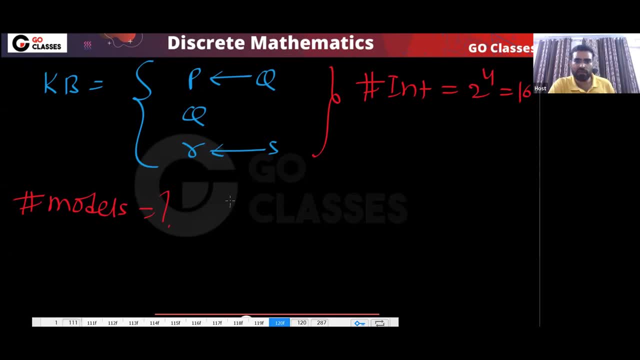 But how many models are there? So you can notice: definitely Q must be true, Q definitely must be true. And you know that if Q is true, then P also must be true. This must be true And remember, Q is already true. 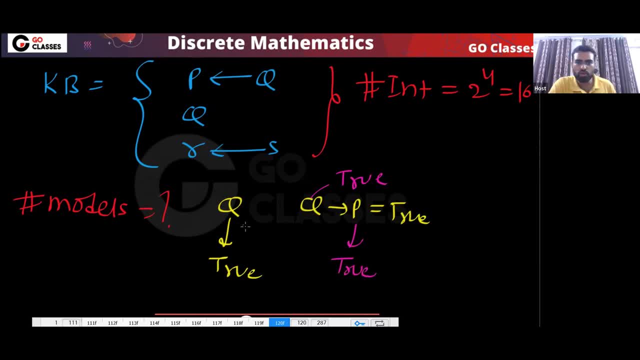 So this P must be true. So for P there is no choice, For Q there is no choice. So I can say for P, Q we only have one choice, It only have one choice And this only have one choice. 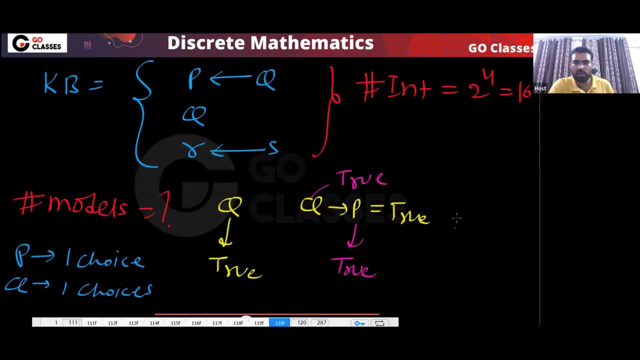 What about R S? For them, we have three choices For R S together. R S together: they have three choices, Okay, Okay, Okay, So the answer will be number of models will be. So I can say number of models that will be 3.. 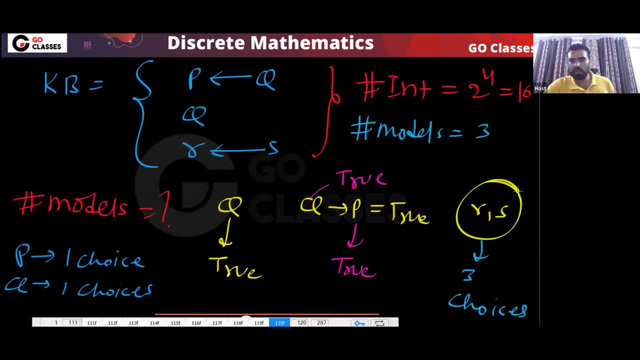 Number of co-models will be 15,. okay, Q can have two choices. No, Q must be true. You have three formula: this formula, this formula, this formula. you have three formula. So Q must be true. If you want model, then this Q must be true. 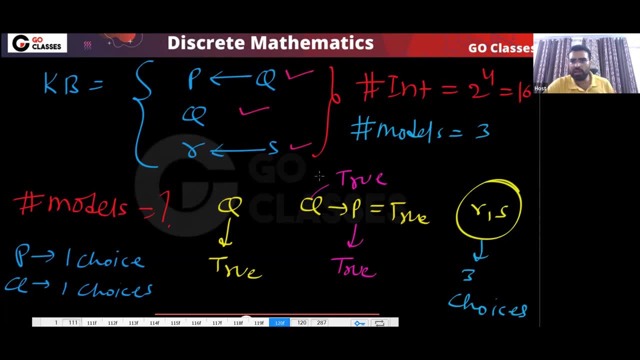 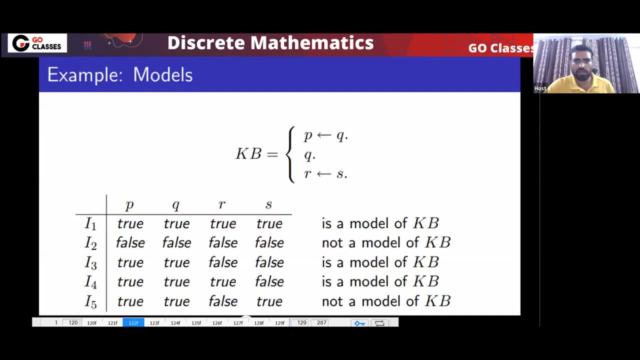 And if Q is true, then automatically P must be true For R S. we have only three choices for R S together, So number of models will be 3.. Okay, let's move on. So I hope all these concepts are clear. 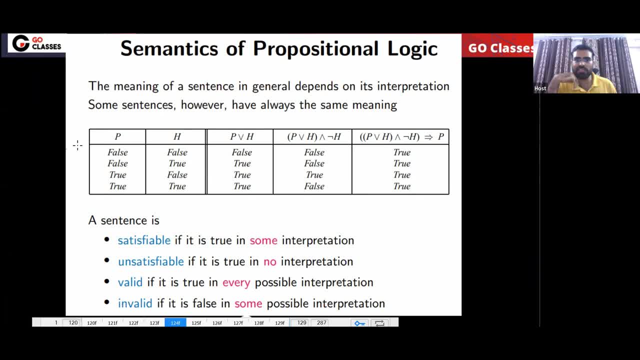 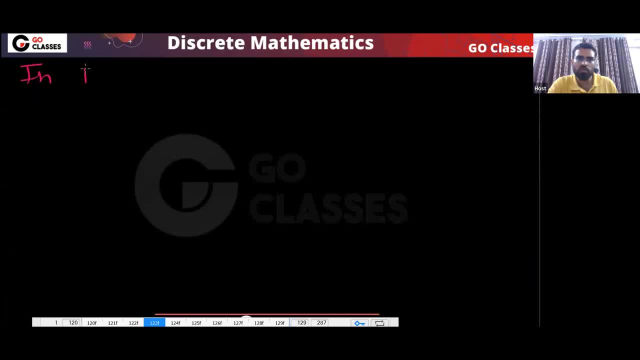 Now, in terms of model, in terms of interpretation, you can define satisfiable. So tell me now what is the definition of satisfiable Now in propositional logic? now you can change the definitions In propositional logic. tell me what is the definition of tautology now. 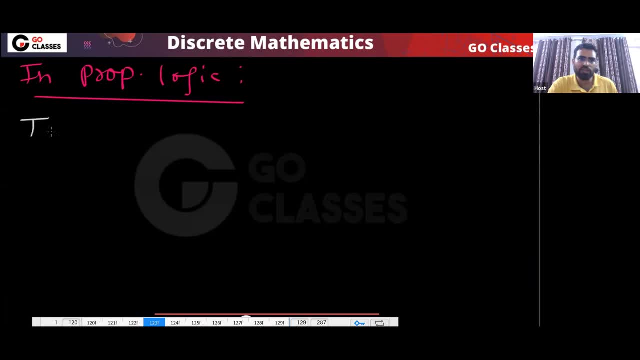 If I ask you what is the definition of tautology now? If I ask you what is the definition of tautology now, If I ask you the definition of tautology, then what that will be. Tautology means for every, every interpretation is model right. 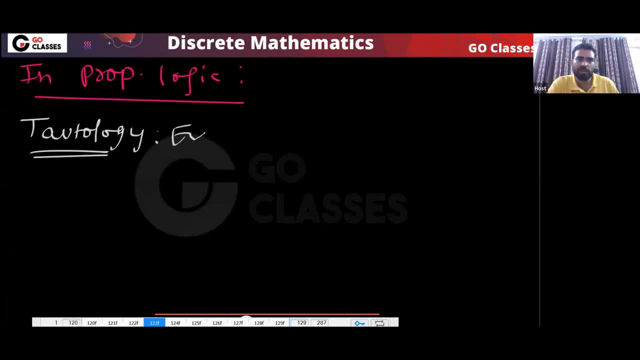 Tautology means every interpretation is model. Tautology basically means every interpretation is model. This is the definition you can use. Every interpretation is model. Every interpretation is model. What can you say about contradiction? what can you say about contradiction? 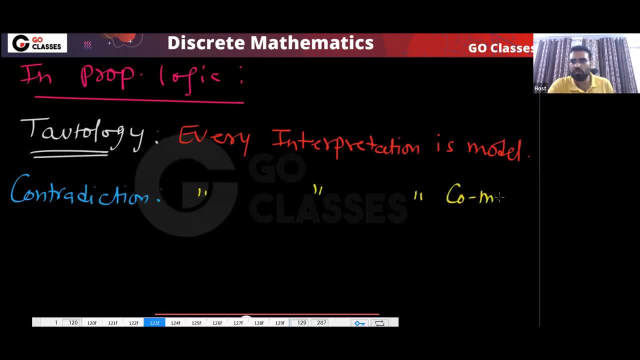 What can you say about contradiction? Every interpretation is co-model, right. Or I can say there is no model. I can say contradiction basically means there is no model. There is no model. Similarly, you can define satisfiable: What is satisfiable? 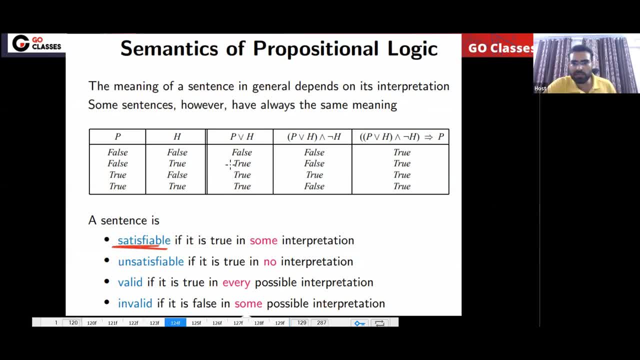 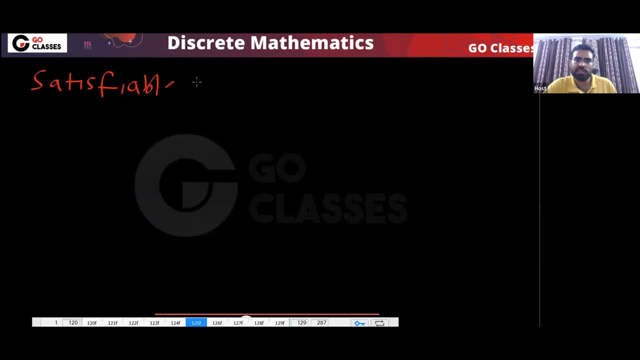 There is some interpretation which is model. There is some interpretation which is there exists a model. Basically satisfiable means there exists a model. Satisfiable basically means there exists a model. And what is the definition of valid? I told you valid and tautology. these are same in propositional logic.